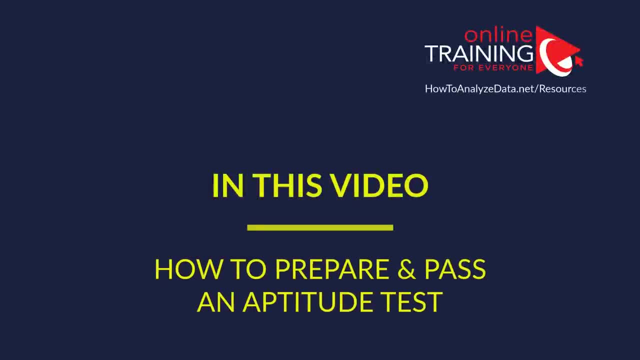 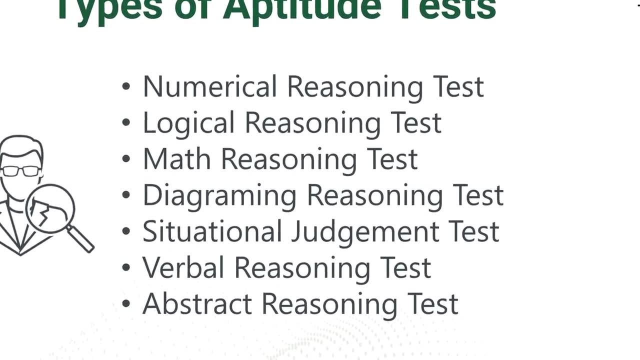 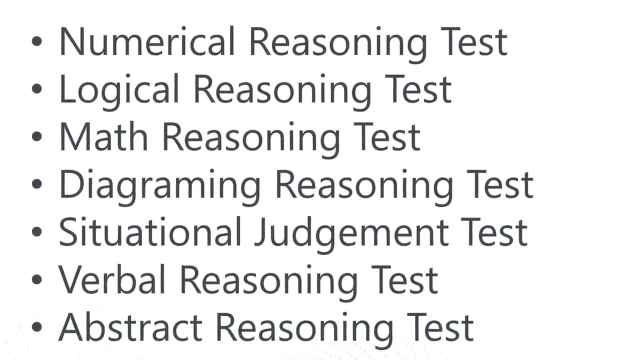 An aptitude test is a pre-employment assessment quiz which is used to determine how well candidate is prepared and how well candidate will succeed on the job. Aptitude test is an umbrella for a variety of different tests. There are various different aptitude tests employers use, based on: 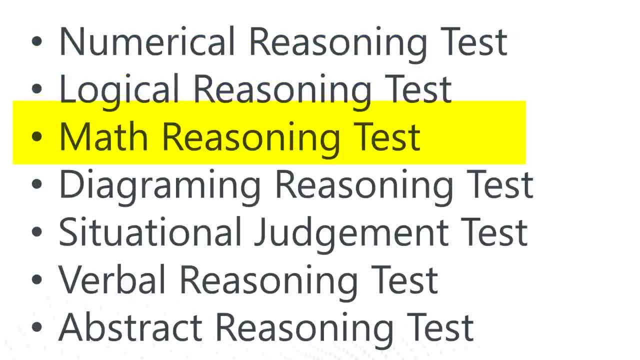 the job candidate might be applying for. Logical reasoning test, math reasoning test, numerical reasoning, diagramming reasoning, situational judgment, verbal reasoning and abstract reasoning test is just another full list of examples of a typical aptitude test. If you're looking for a. 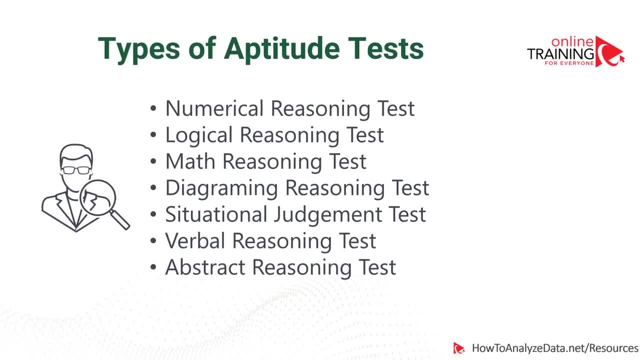 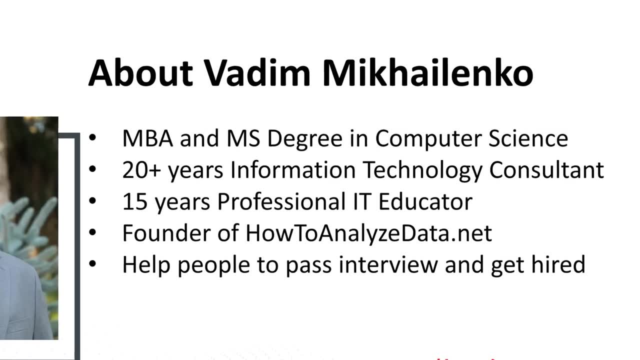 specific test. please make sure to find the relevant video on my channel to get ready and pass the test. Before we move forward, let me tell you a little bit about myself. My name is Vadim Mikhalenko and I have MBA and master's degree in computer science. I have more than 20 years of. 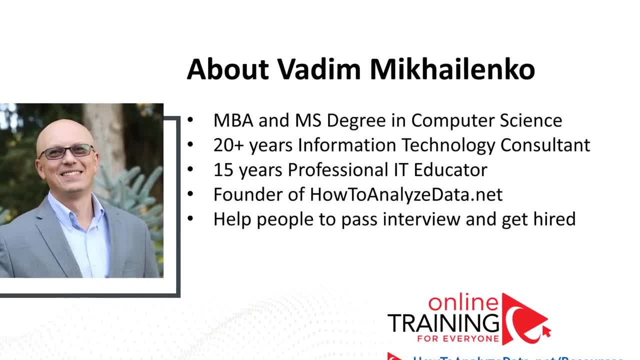 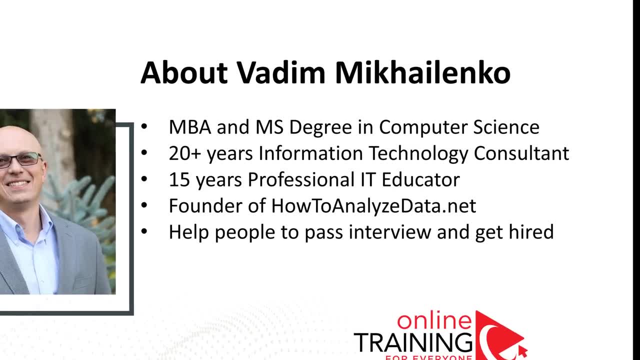 experience in information technology as a consultant and 50 years of experience in the field of computer science. I have a degree in computer science and 15 years of experience as a professional educator. I founded howtoanalyzedatanet website to help people pass the interview and assessment test and get hired for their dream jobs. In this video. 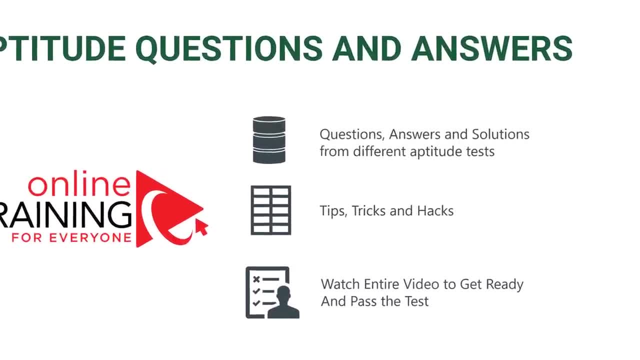 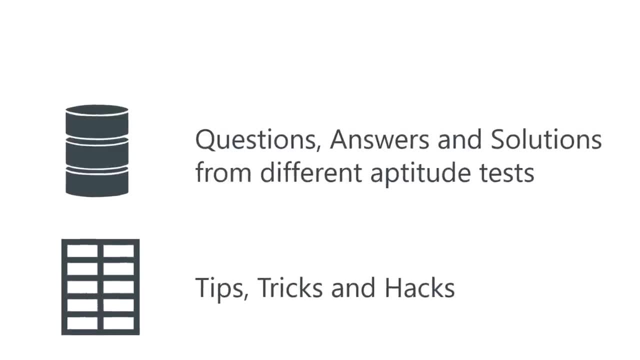 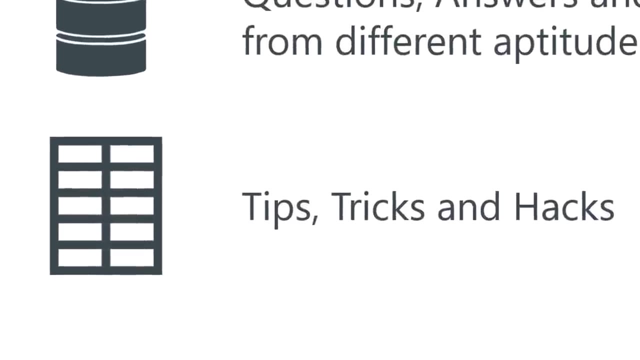 I will show you most typical examples from a different aptitude test, summarizing questions from logical reasoning test, math reasoning test, numerical reasoning test, situational judgment test and abstract reasoning tests. I will also share with you answers, tips, tricks and hacks on how to. 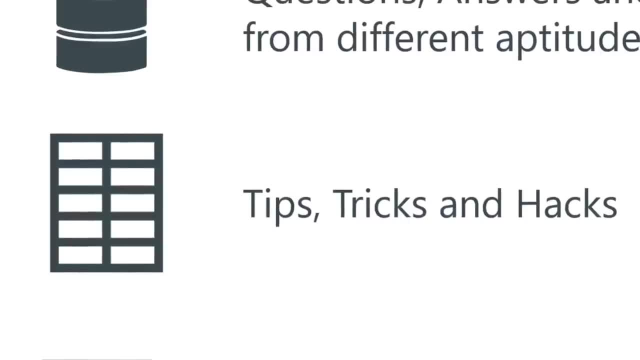 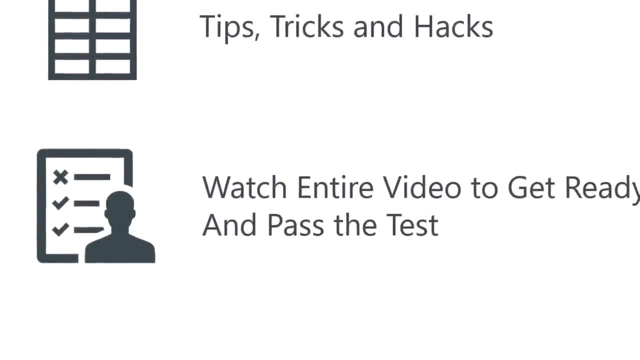 best prepare and pass the test. These questions are in no particular order, so make sure to watch the entire video to test your knowledge and get ready for the test. In this video you will have everything you need to get ready and pass the test. Knowing answers to these questions helped. 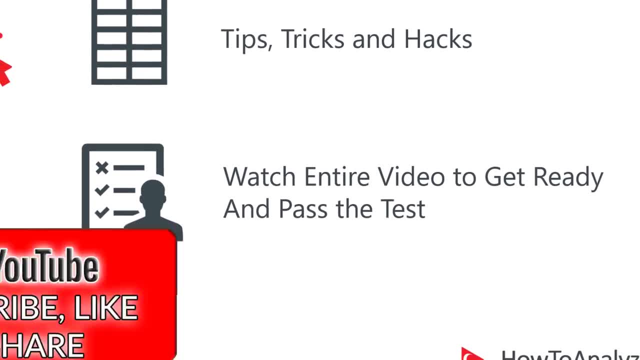 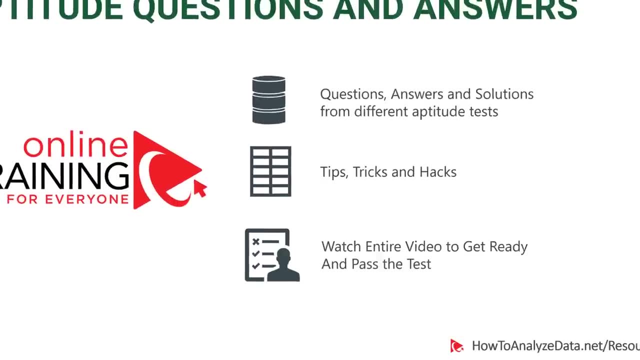 a lot of people and I'm pretty sure it will help you as well. Take a moment and click the subscribe button at the bottom of the screen and make sure to like, share, comment and ask me any questions. I'm happy to answer every question I receive. 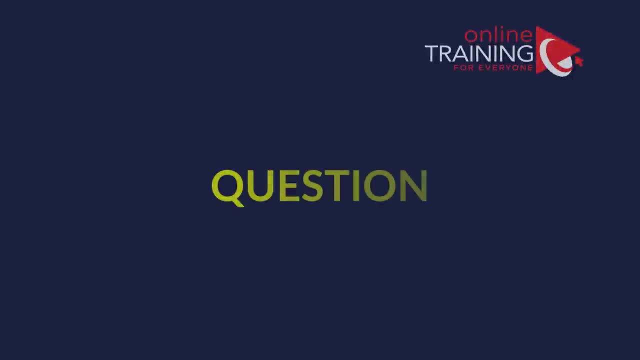 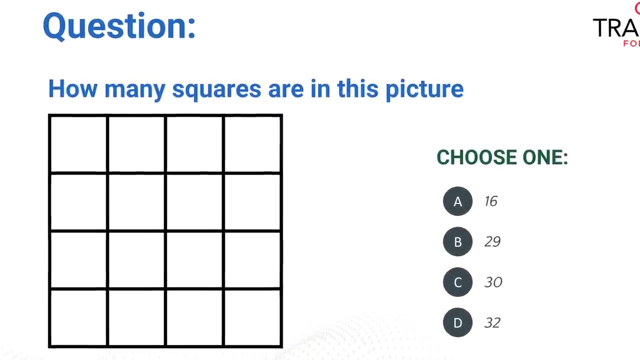 And now let's go ahead and get started. And now let's look at the question which confused tons of people during the test: How many squares are in this picture? And you have choices of 16,, 29,, 30, and 32.. 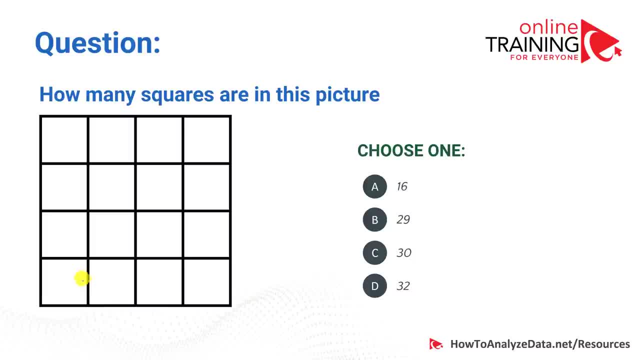 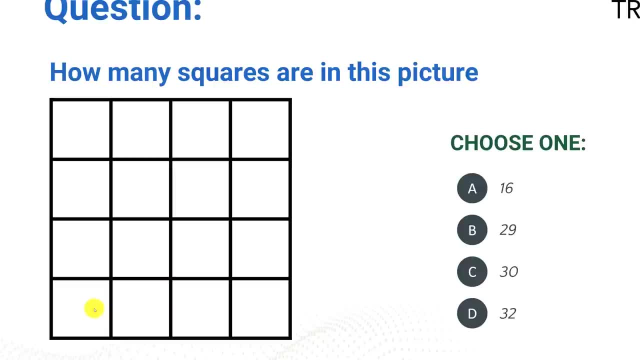 Which one do you think is right? The confusion part of this question comes with the fact that squares are not only the small squares that are shown in the picture. So if you do only small squares, the answer would be 16.. But you can have this area as a square. you can have this area as a. 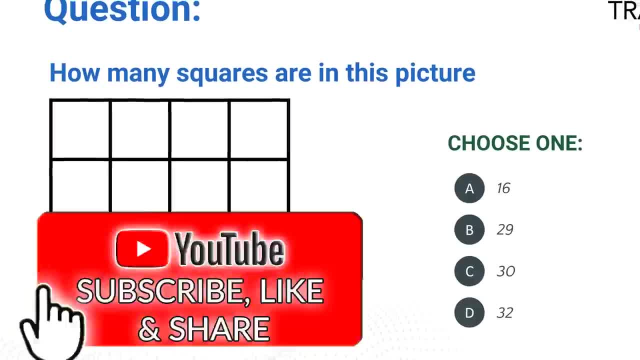 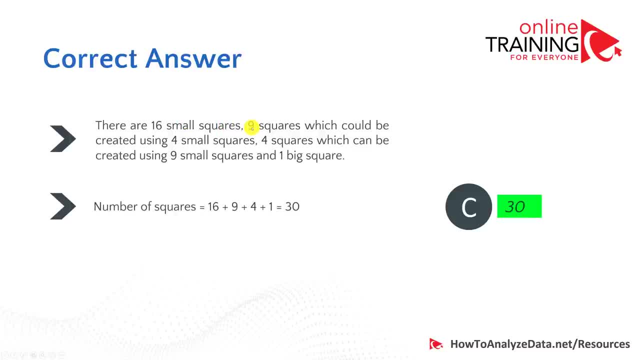 square and large area is also a square. So once you calculate all of those, you will get to the correct answer, And the correct answer is 30, because there are 16 small squares, 9 squares which would be created using 4 small squares, 4 squares which can be created using 9 small. 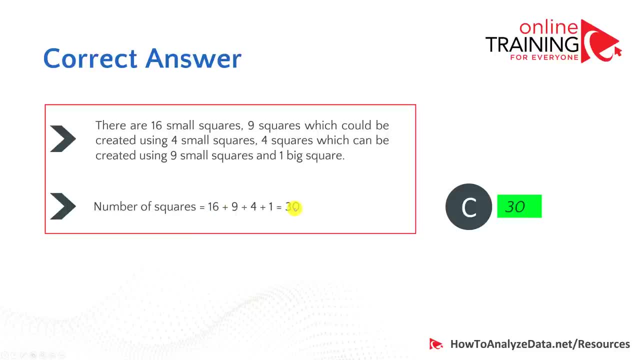 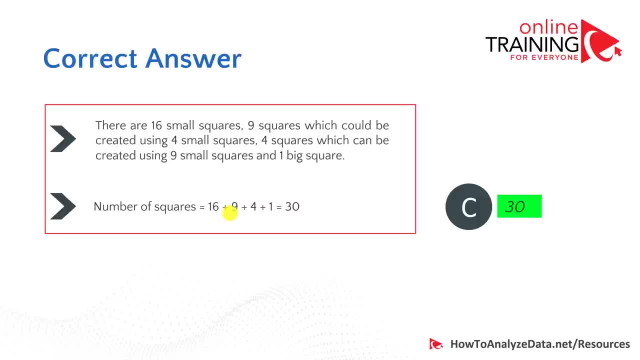 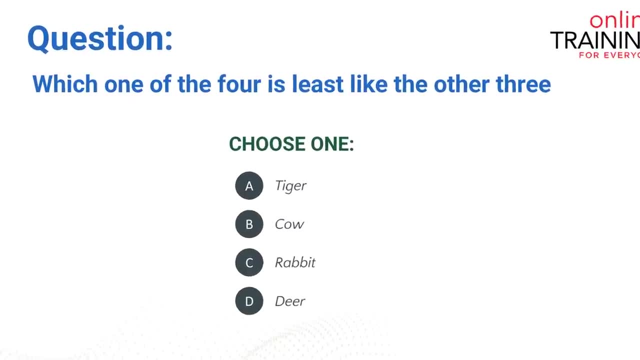 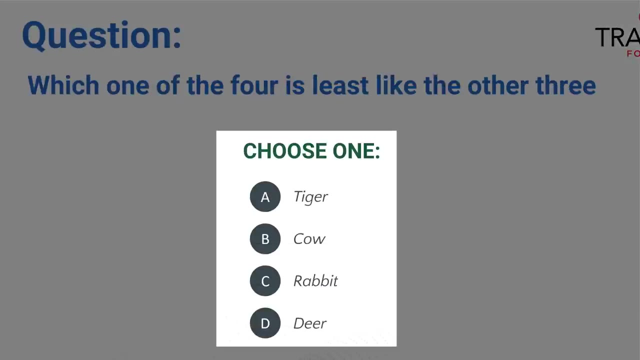 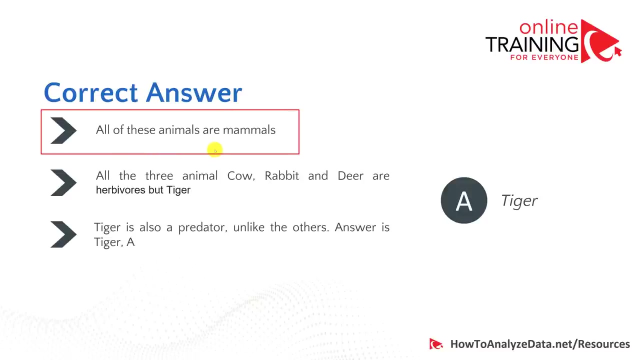 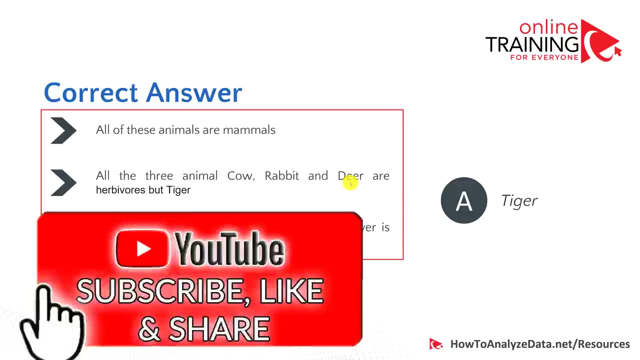 start with the answer 30.. So let's start with the answer 30.. So let's start with the answer 30.. So let's. tiger is a predator, So the correct answer is A, which is tiger. So hopefully you've got this one. 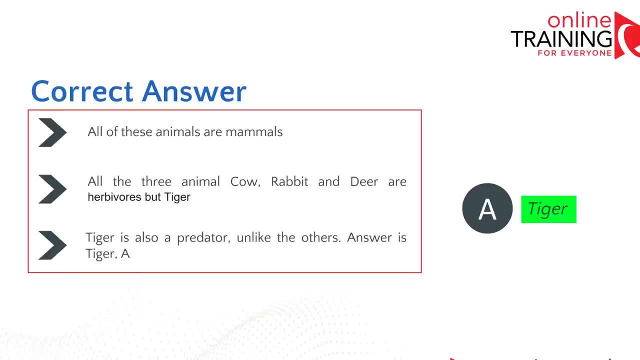 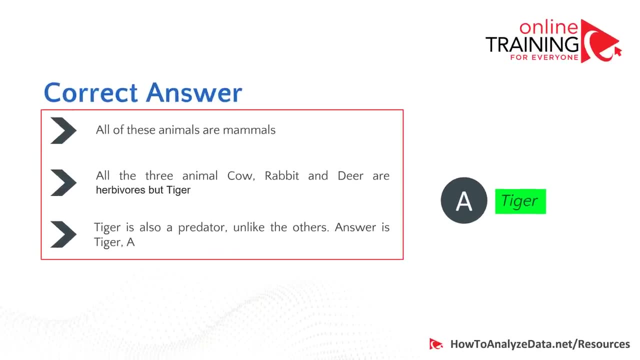 right. It's a tricky one and it tests your knowledge of exclusion, meaning that you need to read the test question correctly and then you need to find out the correct choice. Hopefully you've got this one right. I'd like to ask you to participate in our daily Excel assessment test. 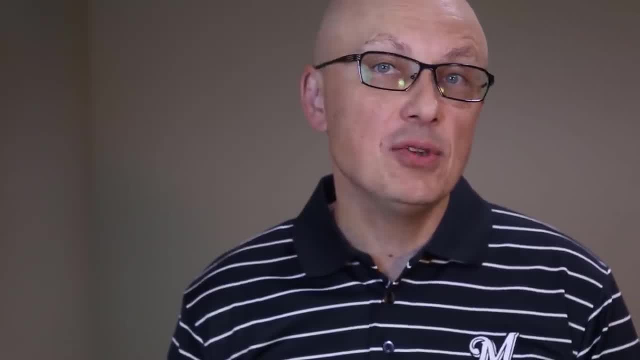 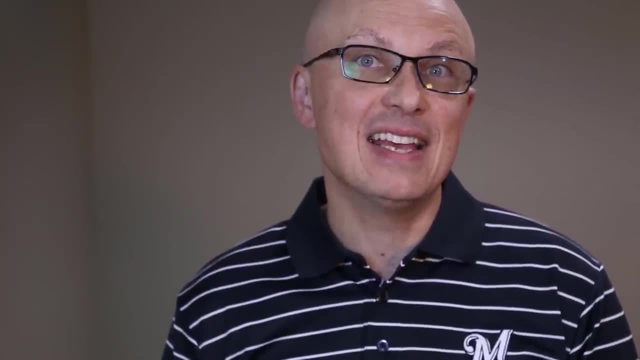 challenge. I post new questions every day in the community tab of this channel and give you an opportunity to answer this and try it, And I post the answer in the comments next day. So please make sure to check it out and test your knowledge. And now let's continue and get you ready for the. 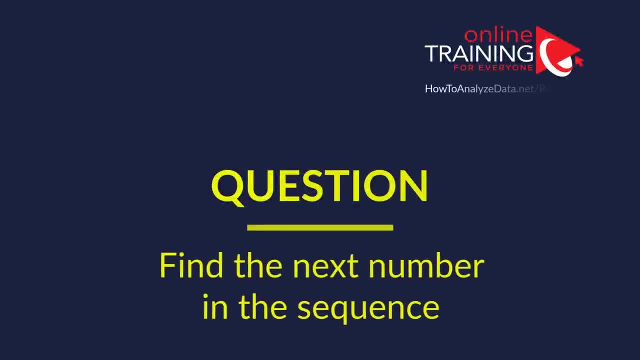 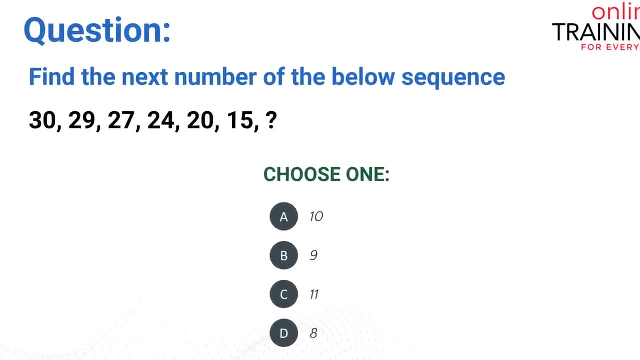 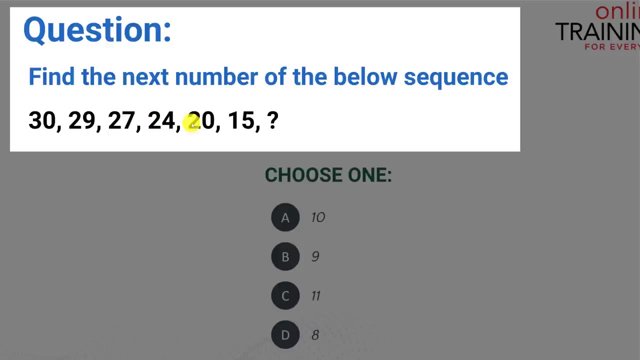 test. So here's the question which is frequently used as part of numerical reasoning and logical reasoning tests. Find the next number of the below sequence And you have series of numbers: 30,, 29,, 27,, 24,, 20,. 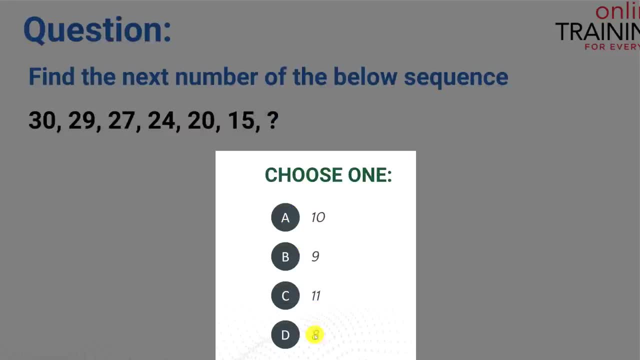 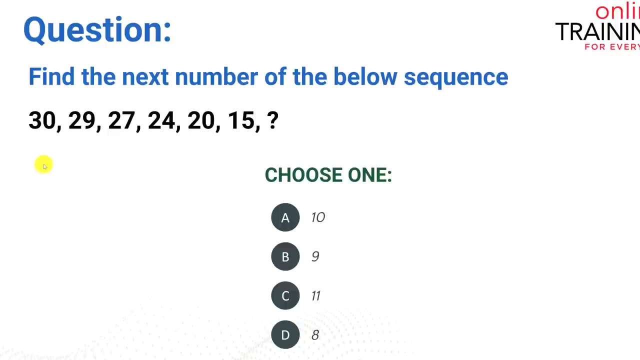 15, and you have choices, four different choices: 10,, 9,, 11, and 8.. Which one do you think is right, And how would you even approach answering something like this, The key to answer something like this: 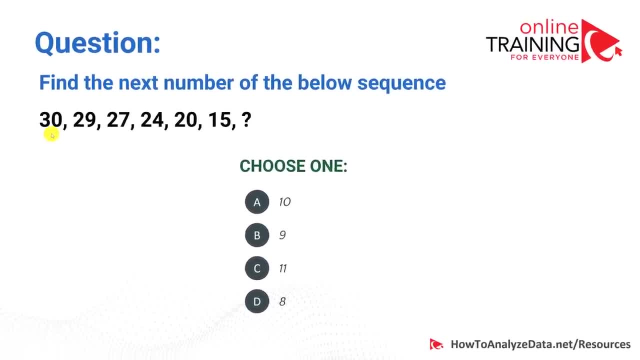 in this types of questions in general is to detect the pattern. So you see, the pattern here is you increase the number every time you go from one number to the next. 30 is one more than 29, and 27 is two more than 29.. 24 is three more than 27.. 20 is. 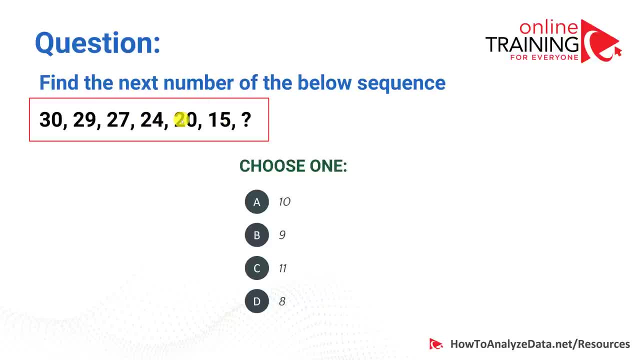 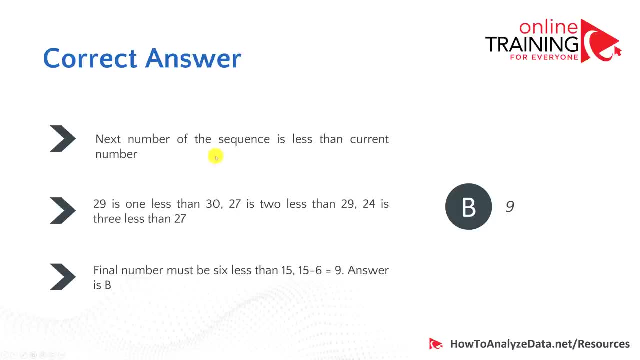 4. More than 24.. And 15 is 5 more than 20.. So the next difference would be 6, and 15 minus 6 would be 9.. Let's recap: So next number in the sequence is less than the current number. 29 is less than 30.. 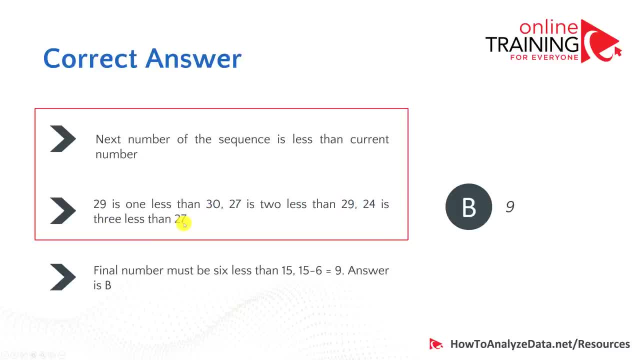 27 is 2 less than 29,, and 24 is 3 less than 27.. And you can continue the sequence once you detect it. And final number must be 6 less than 15, which is 9.. So the correct answer is B, which is 9.. 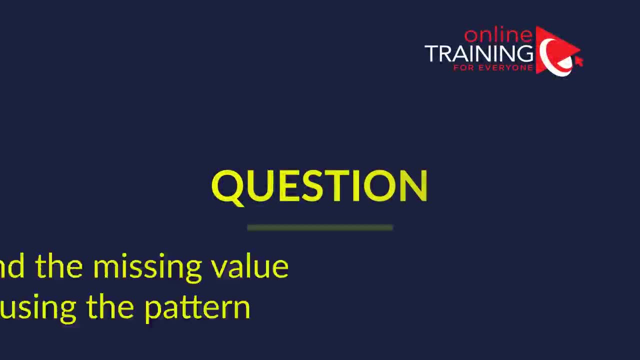 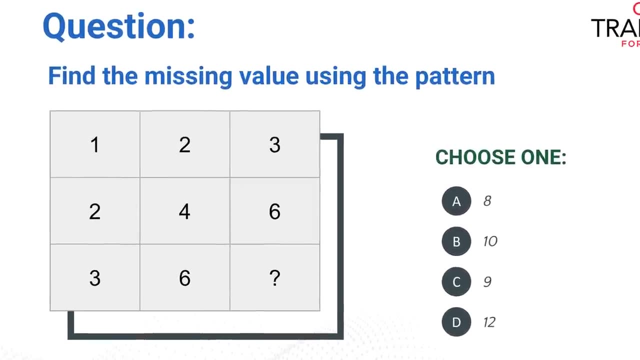 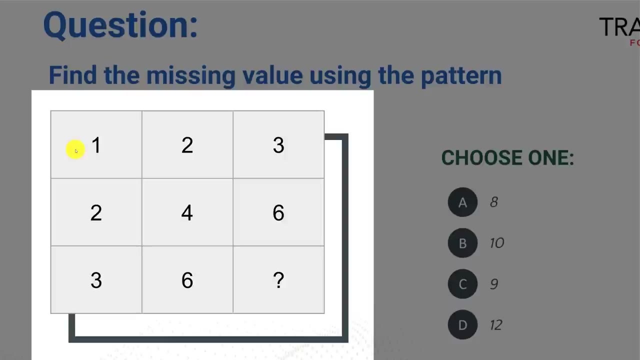 Hopefully you've got this one right. Now let's look at the question: find the missing value using the pattern. You see the three by three box and one of the values in this box is missing. So what is the pattern? And there are four choices. 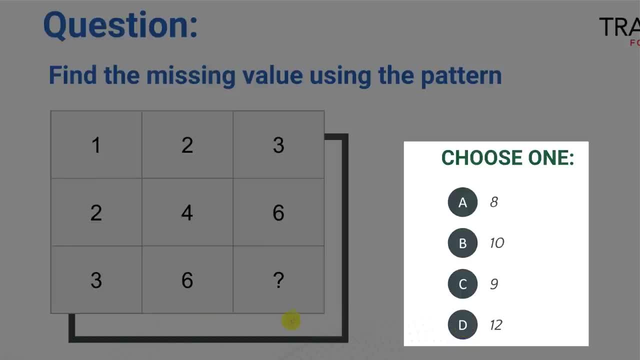 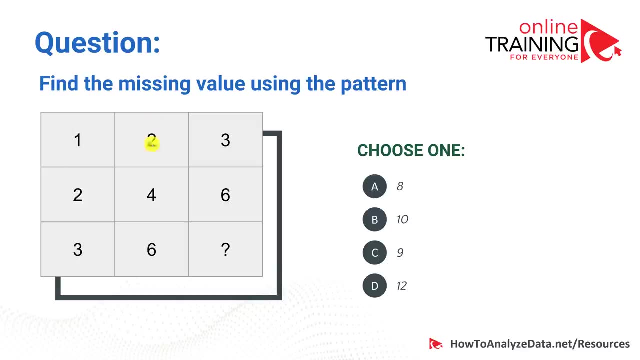 We have A, B, C and D right, And obviously you would have to find the pattern and calculate the value. So what do you guys think is the right answer here? Before I reveal the right answer, let me try to discuss with you the pattern. 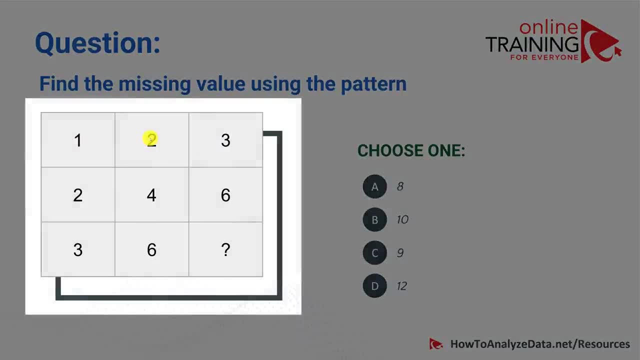 So you see one, two and three, right, But then this one, two, four and six. So it's not sequential. So it's not like you go: one plus one equals two plus one equals three. There is a different type of pattern here. 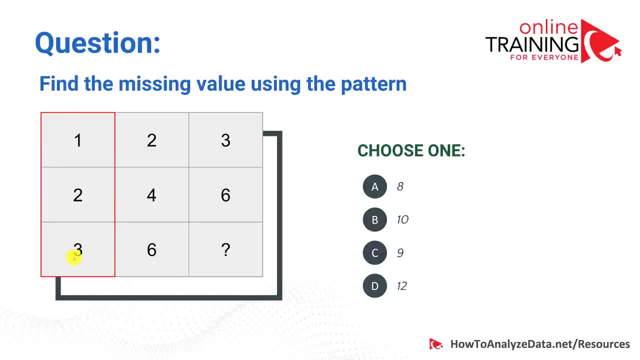 And the right pattern here is that one plus two equals three, right, And then two plus four equals six, And once you know the pattern, you can easily calculate that three plus six equals nine. So the right answer here is choice C. Let's validate. 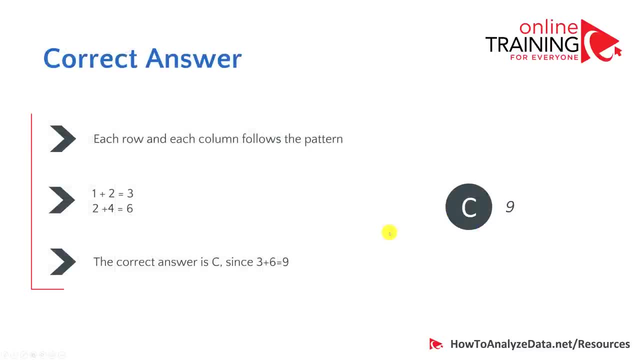 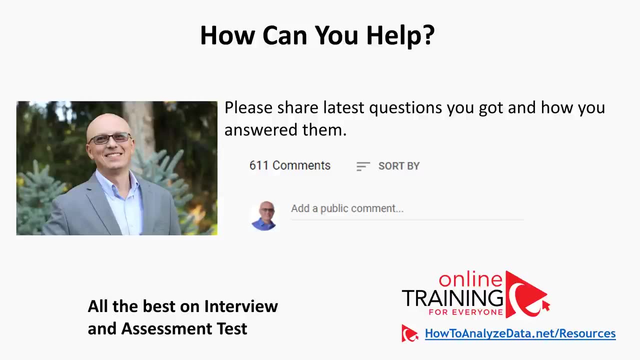 And you're absolutely right. The right choice is choice C, And this is exactly the logic that I just presented to you. Hopefully you've got this one right. A lot of you are interested in asking me: how can I help others? One of the ways you can help other people. 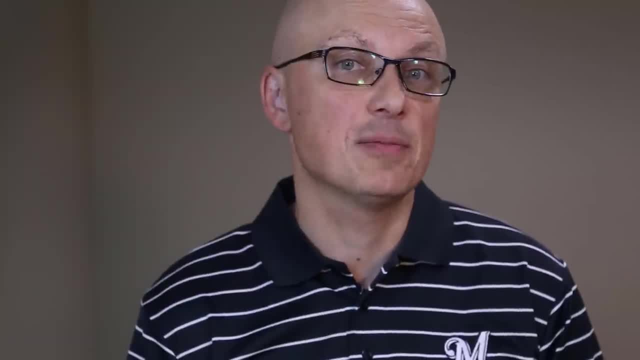 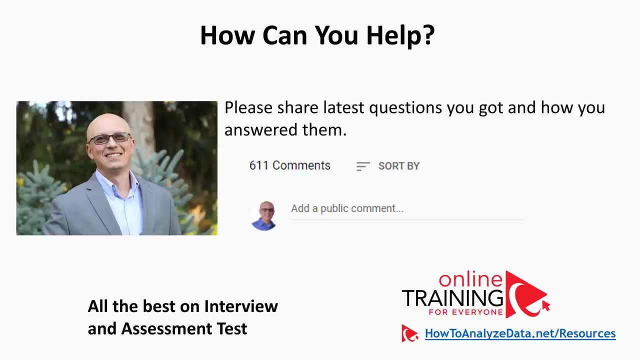 is by sharing the latest questions that you see on Excel interview and assessment test and how you answer them. Please share the questions you recently encountered in the comments section. If you know the answers, please share them as well. And now let's continue and get you ready for the test. 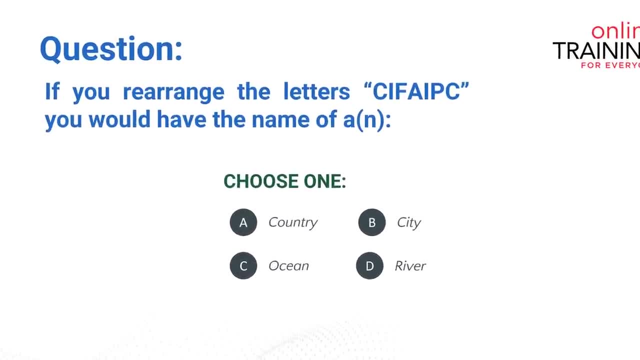 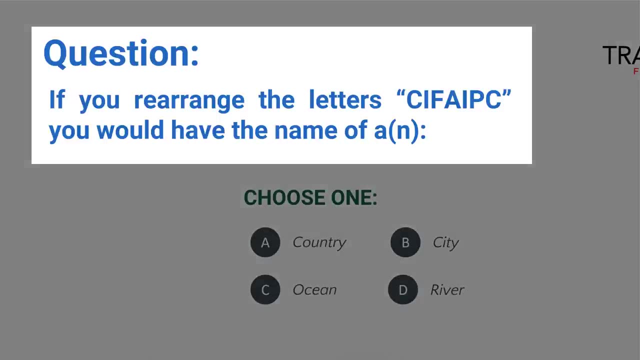 Now let's look at the question which is frequently used as part of verbal reasoning aptitude test and psychometric tests. If you rearrange the letters C-I-F-A-I-P-C, you would have the name of an and therefore choices. 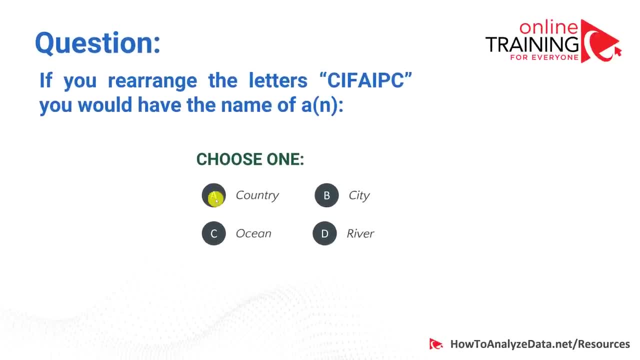 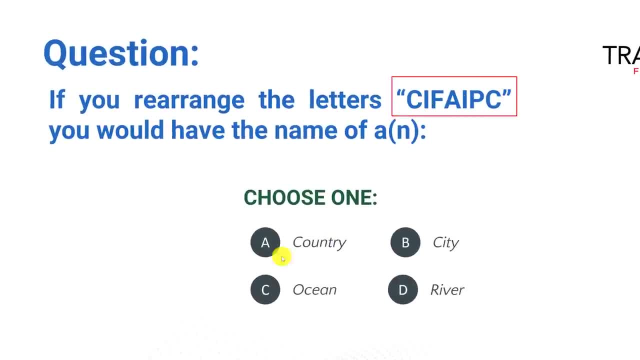 You can't rearrange this set of letters to get to the country. You can't rearrange it to get to the ocean letter or to any one of these letters. It is country name that would be a result of this rearrangement, or ocean name that would be or city name or river name. 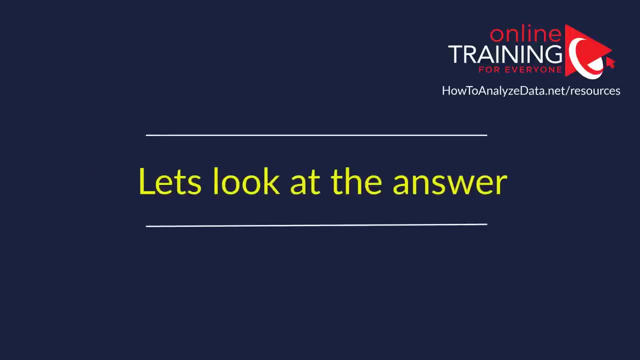 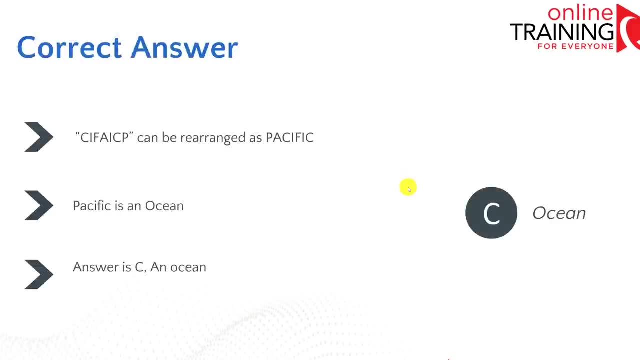 So let's see if you can get this one correctly. Unfortunately, there is no easy way to prepare yourself for these types of questions, And the correct answer here is Pacific. So the answer is Pacific Ocean, right, But there's no way for you to know this. 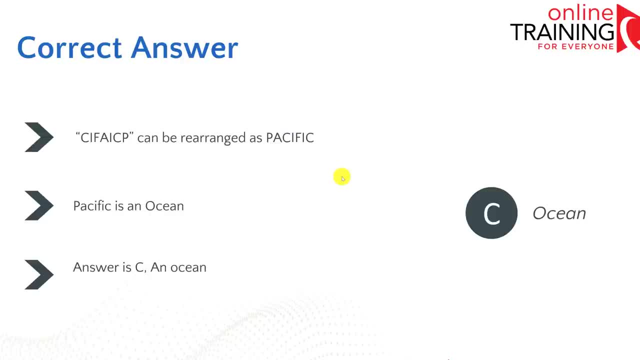 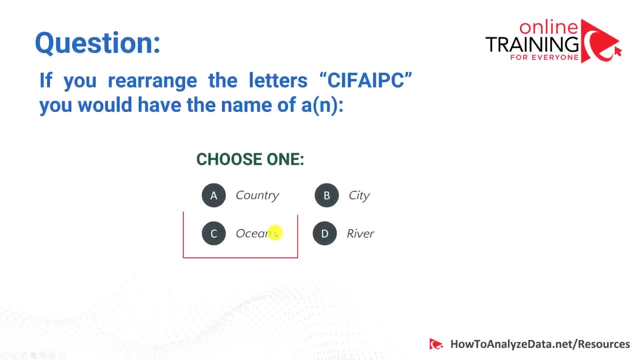 You've probably heard the term of Pacific Ocean, but the best practice to answer these types of questions would be to go and start with the smallest one, And smallest one would be ocean. There are only very few oceans, and you're probably much better off starting and going. 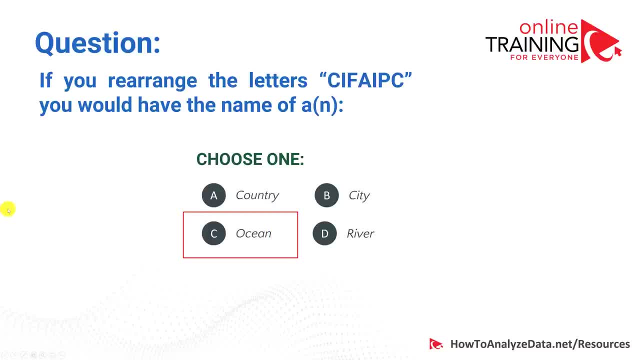 and counting through all these oceans that are available, And one of those oceans is the Pacific Ocean, Because if you start to go with city, river and country, there are too many countries, too many cities and too many rivers, And the expectation is that you would not know all of this. 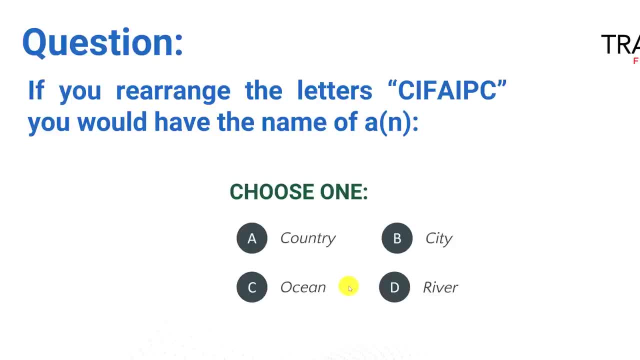 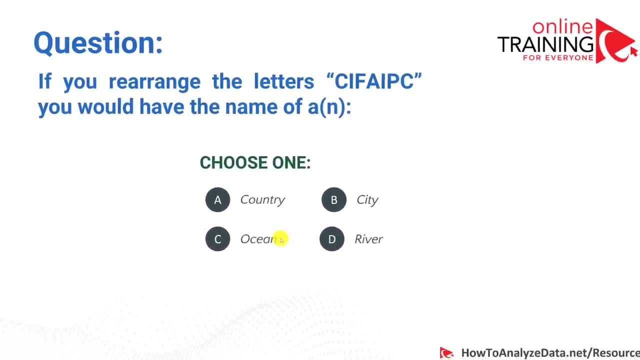 and you can't answer. So that's the best way to come to these questions: Identify what is the smallest number of items that's on the list and then loop through these items to identify the right one. So going back is Pacific Ocean is the answer. 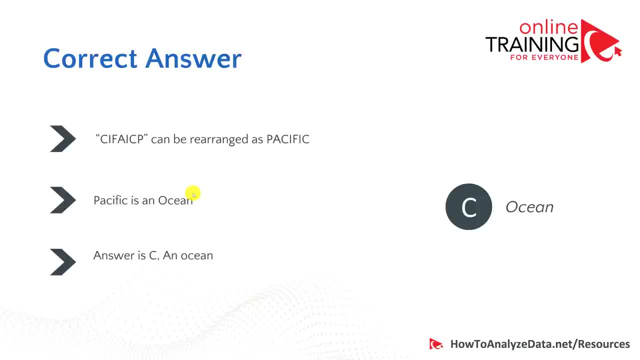 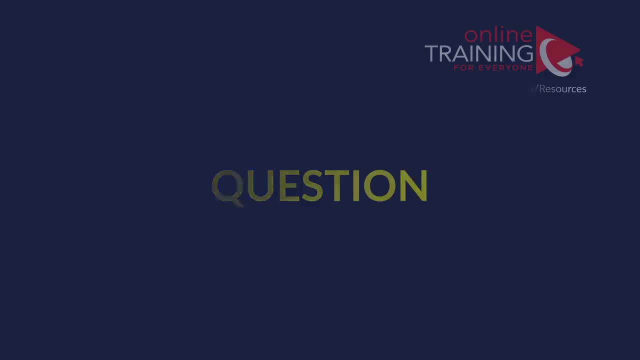 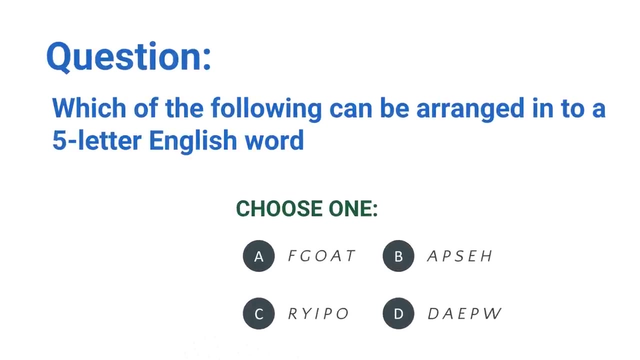 And hopefully you will have the tips and tricks to get these types of questions correctly. Now let's look at the question where you test it not just how well you know English, but also how well can you operate with the letters and take guesses based on the questions asked. 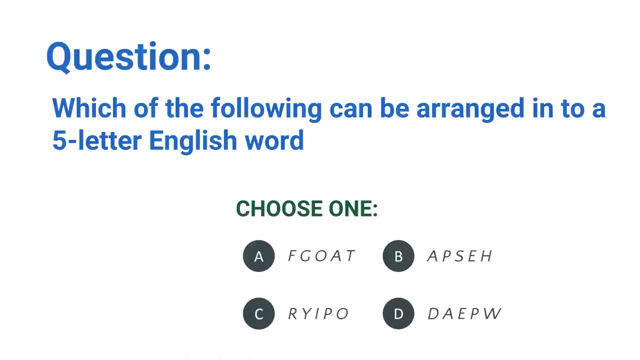 A lot of times these types of questions used in the verbal reasoning tests and in a lot of other tests as well, For example psychometric tests or logic reasoning tests. these types of questions we see all the time. So the question: Which of the following can be arranged? 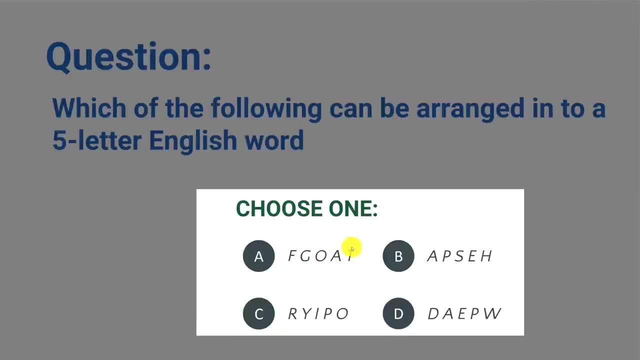 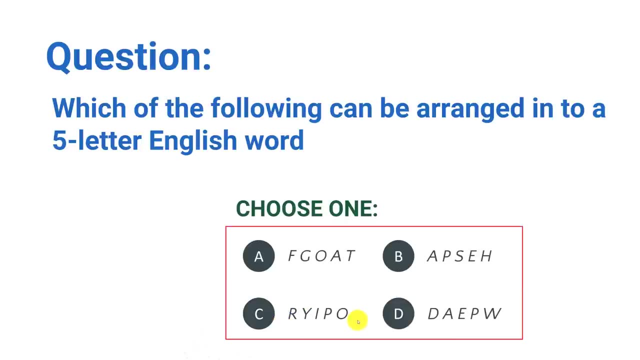 to a five letter English word And there are four choices with five letters of the words And you kind of would need to look at each choice and you would need to take a guess which one would be the one which leads to specific English word. 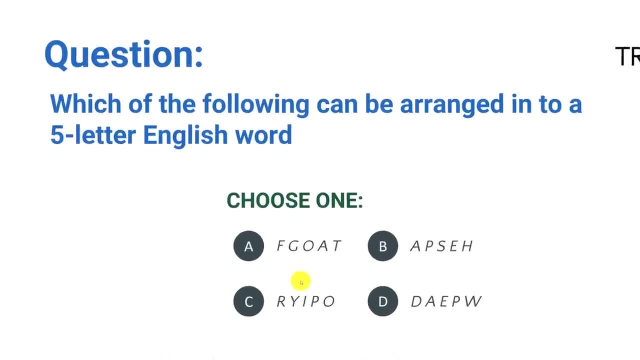 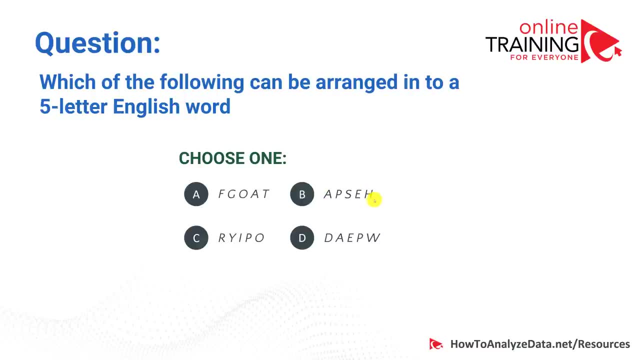 And obviously nobody gives you the English word, So you would have to take a guess in the word and combine these letters So they will be represented by the specific English word. So which one do you think is the right choice? A couple of suggestions here. 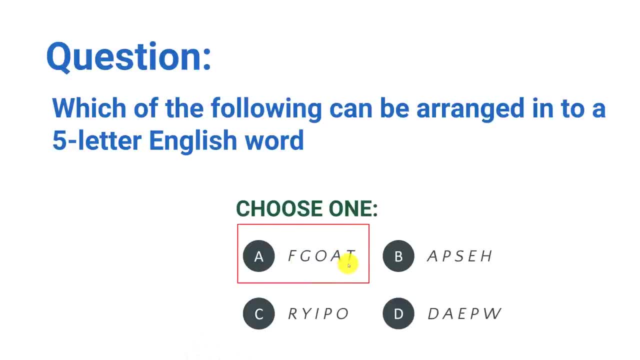 You see, choice A has inside of this letters English word goat. So typically it's the wrong choice because typically you wouldn't be able easily rearrange this word into something else. Typically- and again it's only typically- but you would want to start with the letter. 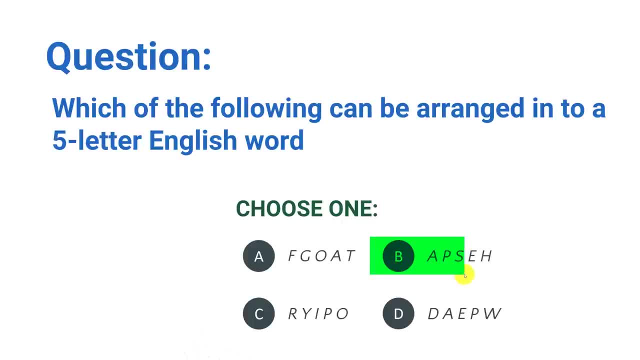 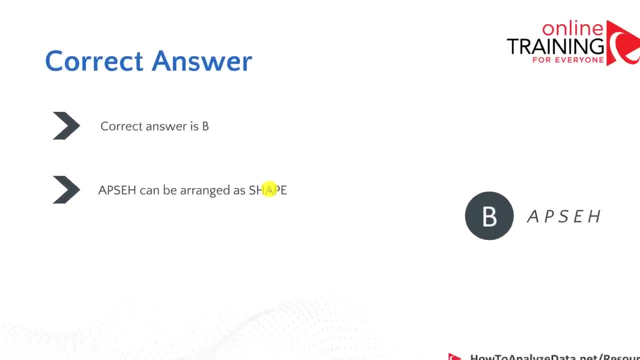 somewhere in the middle, And the right choice here is choice B, And it's the word shape. That's really the word that the end result of it. You don't have a way of knowing Because you don't know what the end word is. 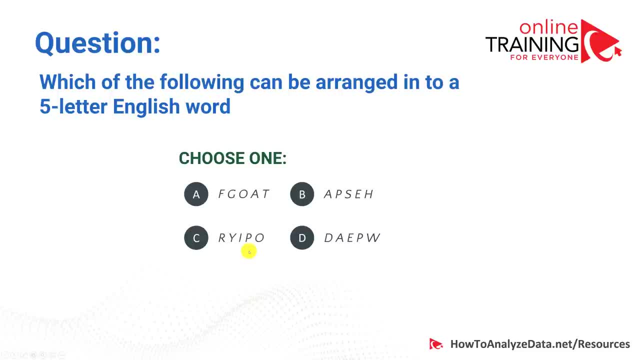 So you would have to look realistically at all the different choices and see if you can combine them. But I would start with the middle letter, because typically they try to trick you And first letter is typically not the one that starts this new word. So find more exercises like this. 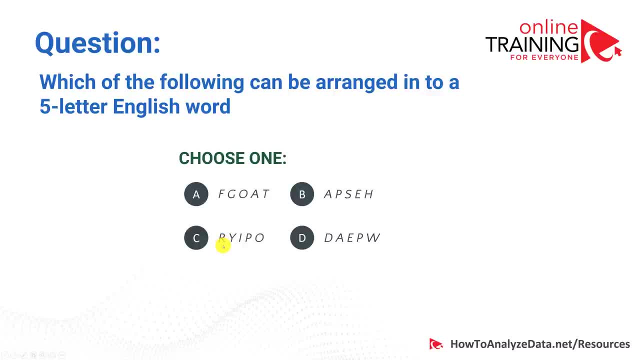 This one was tricky, This one was difficult. Very few people guess it right, But it takes practice to get these types of questions correctly. So make sure Google or find on the internet these types of verbal reasoning questions and see if you can get better at this. 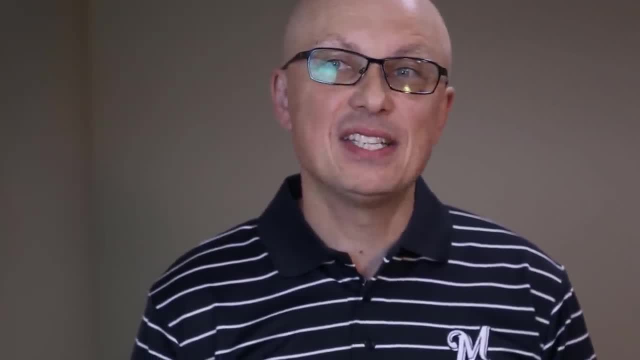 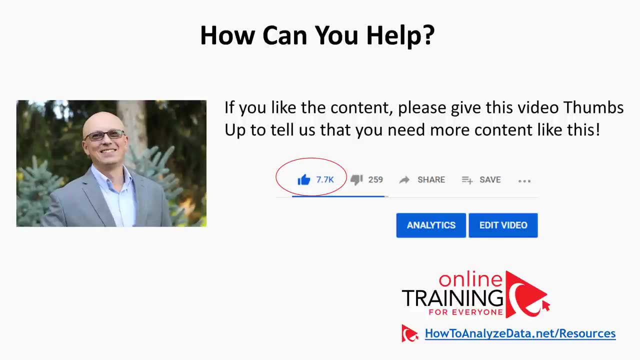 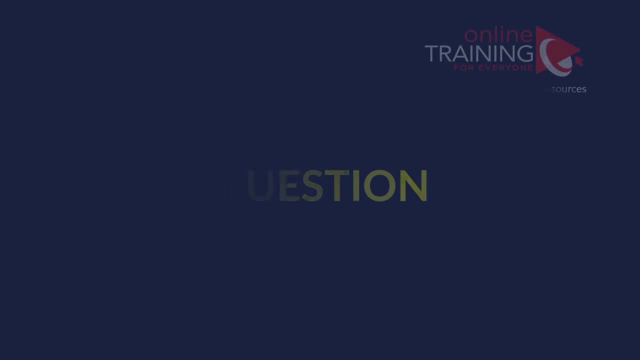 Can I ask you to do me a favor? If you like the content, please give this video a big thumbs up to tell us that you need more content like this. And now let's continue and get you ready for the test. Let's look at the question. 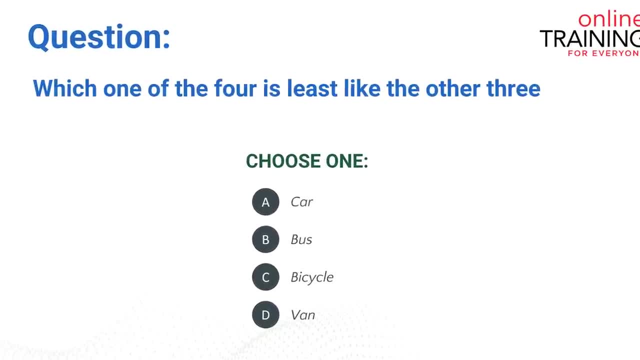 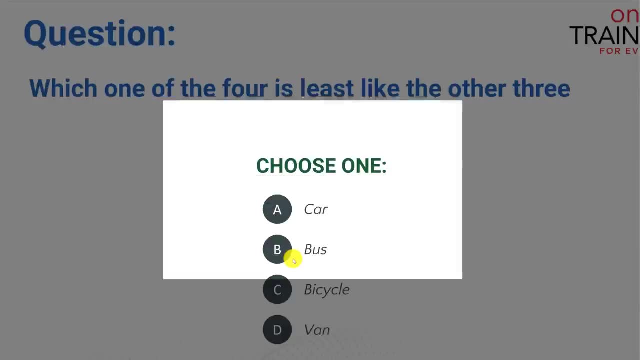 which tests your knowledge of logical reasoning, which is very frequently used as part of psychometric tests And aptitude tests. Which of the four is least like the other three? And you have four choices: car, bus, bicycle and van? 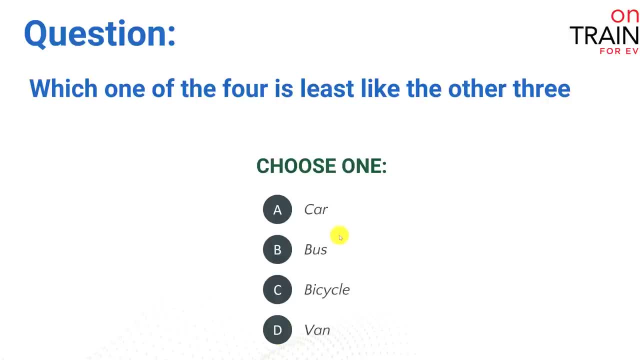 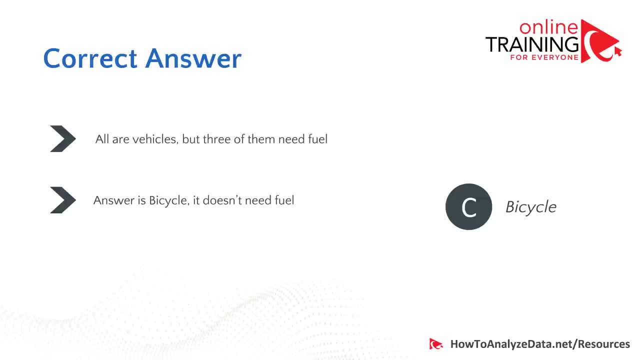 Multiple different options here. You can arrange all these items by size, by weight or maybe by something else. Do you think you know the answer? And, as you might've figured out, the correct answer is C, which is bicycle, Because all of these four choices are vehicles. 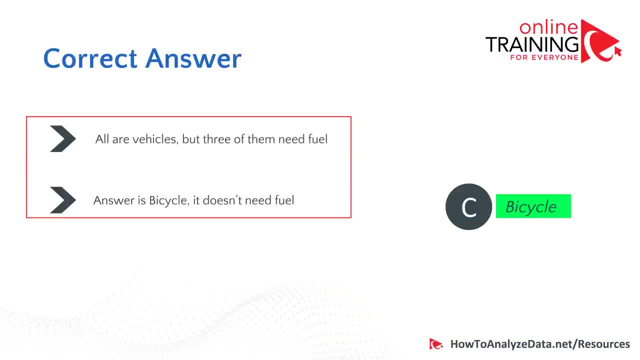 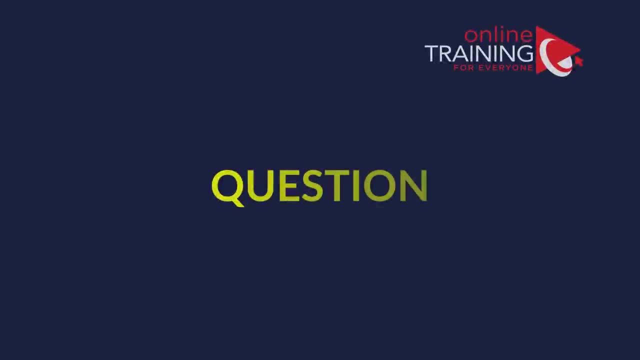 but three of them need fuel. So answer is the bicycle which doesn't need fuel, which is not, like you know, like a bicycle, Like all of the others. Hopefully you've got this one right. So here is the tricky question. 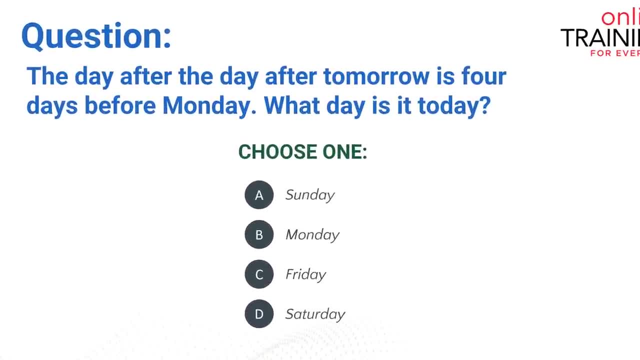 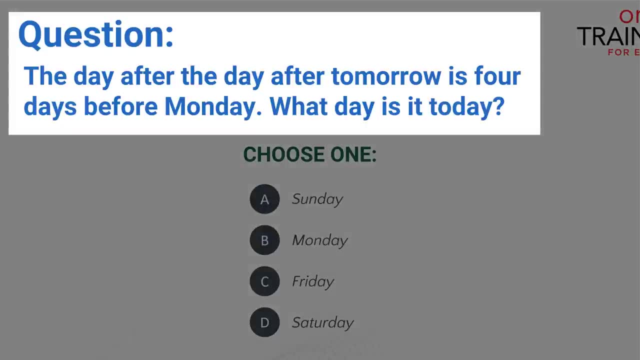 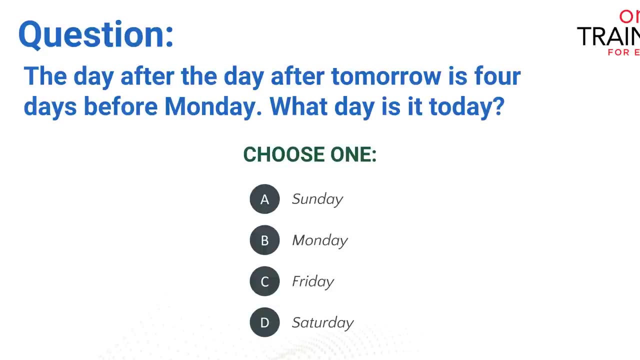 which is frequently used as part of logical reasoning tests and numerical reasoning tests. The day after the day after tomorrow is four days before Monday. What day is it today? And you have four choices: Sunday, Monday, Friday and Saturday. And the reason I'm laughing is because this tells me. 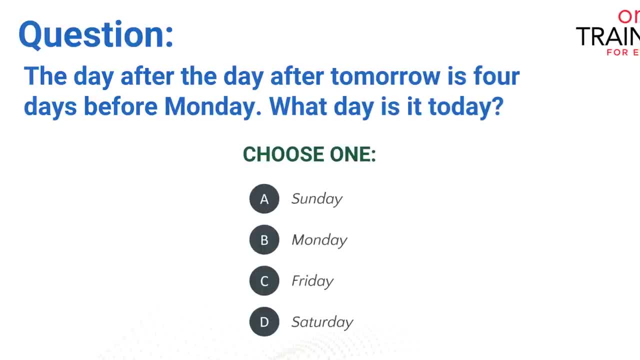 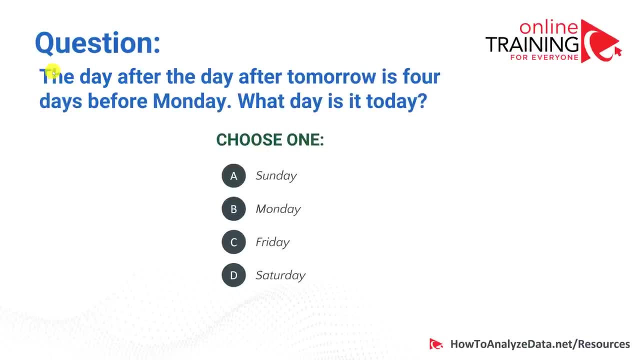 that you always should come to those types of tests after a very good night's sleep and try to schedule them in the morning. That's the best advice I can give you, Because sometimes, if you come to this type of test tired, you wouldn't even understand what they're asking you to do. 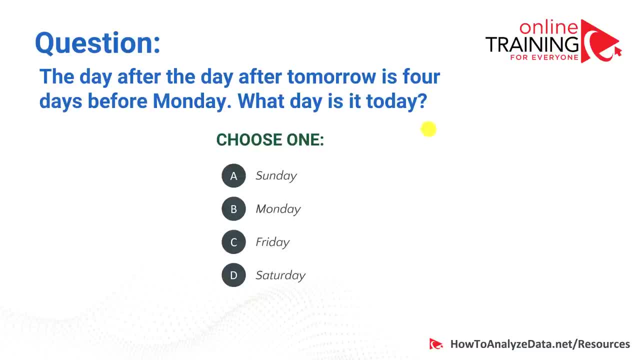 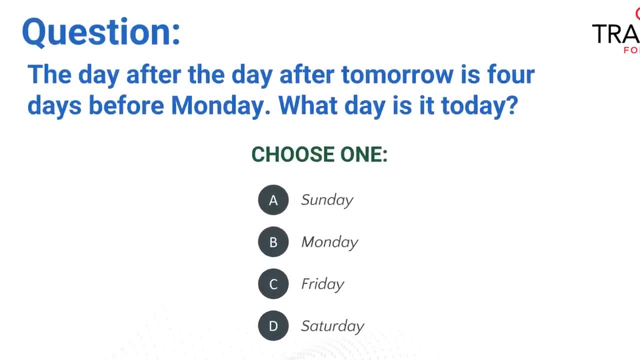 So do you have an idea how to answer this? Let's take a look at the answer Again. most of the time, you have to use reverse method to get to the right answer, And the reverse method tells us that four days before Monday is Thursday. 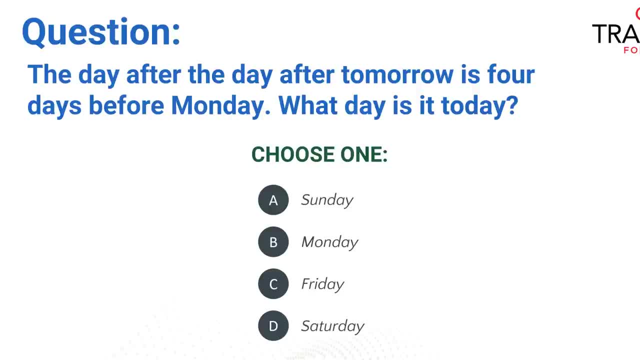 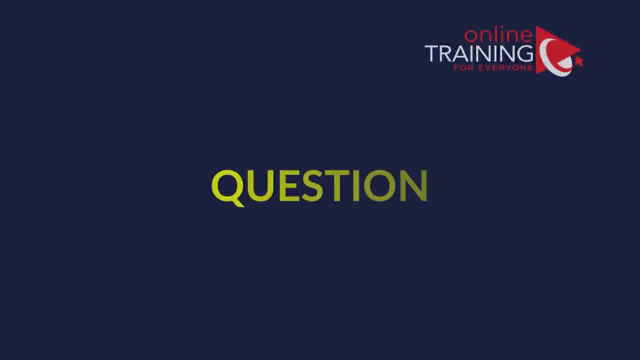 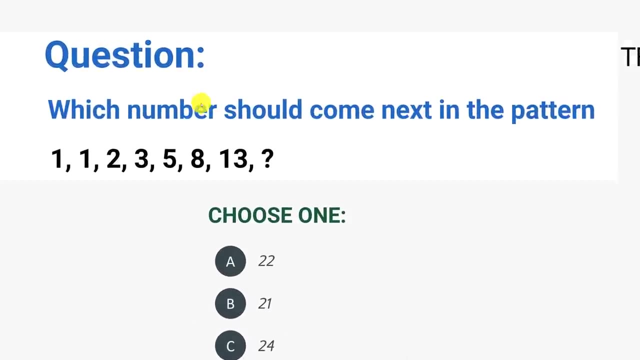 And day before day before Thursday. Thursday is Tuesday. If tomorrow is Tuesday, today is Monday, So the correct answer is B, Monday. Hopefully you've got this one right. Now let's look at another pattern type question. Which number should come next in the pattern? 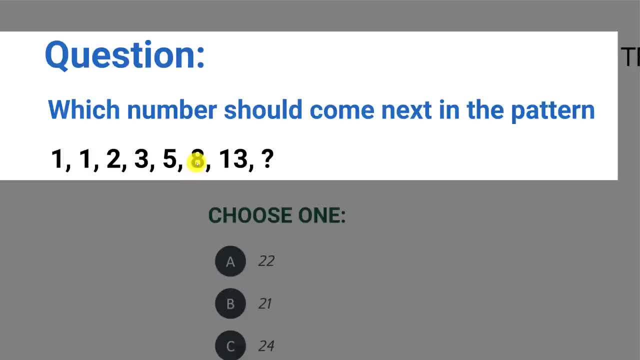 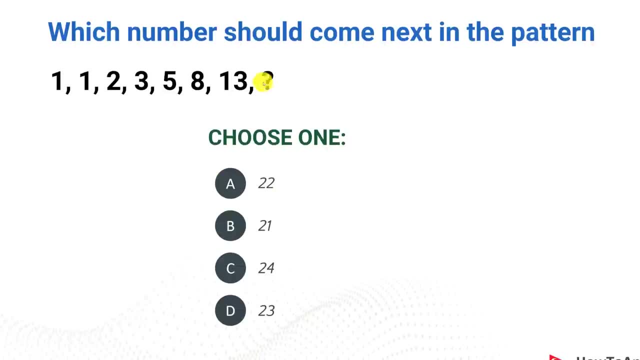 And then you have pattern of numbers One, one, two, three, five, eight, 13.. So let's first determine what's the pattern here. Obviously, there are four choices, but the result here is calculated Based on the pattern that we would need to determine. 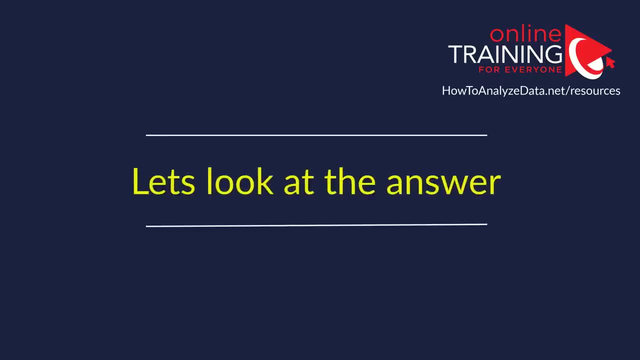 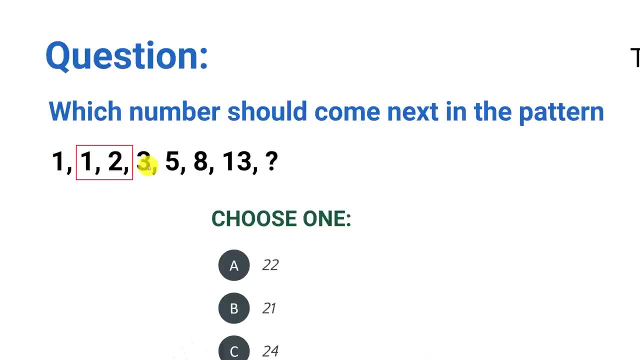 Which one do you guys think is the right one here? Well, let's look. So we have one one, and then one plus one equals two. Then one plus two equals three. Then we have two plus three equals five, And then you can kind of keep going. 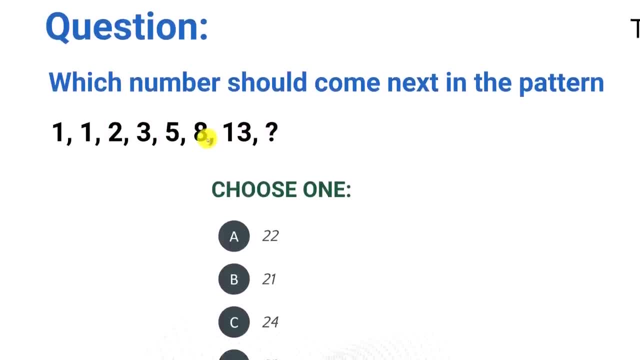 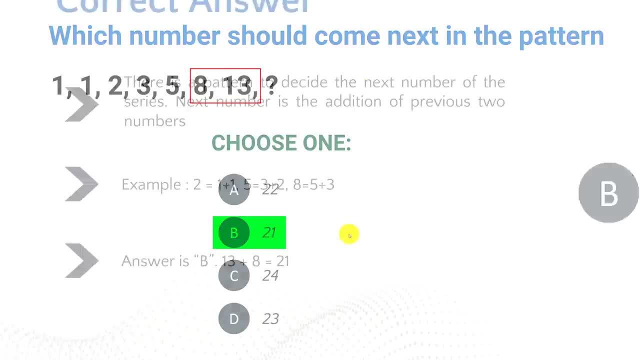 So to calculate the next number, it's basically the sum of the previous two numbers. So eight plus 13 is 21.. So the right choice here is choice B, which is 21.. And this is the explanation That the pattern here is really the sum. 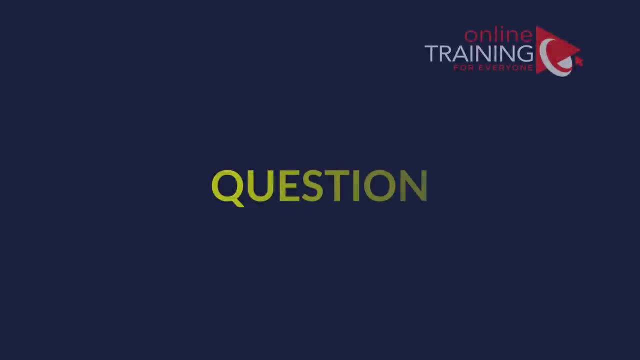 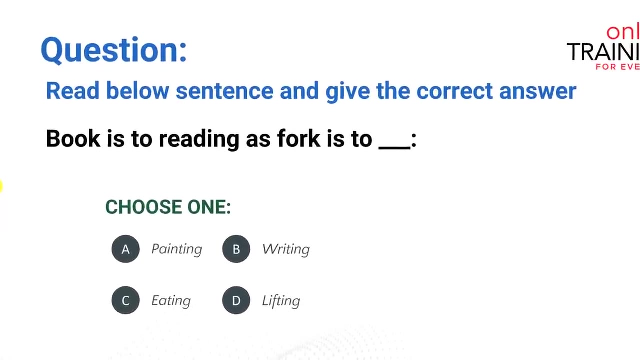 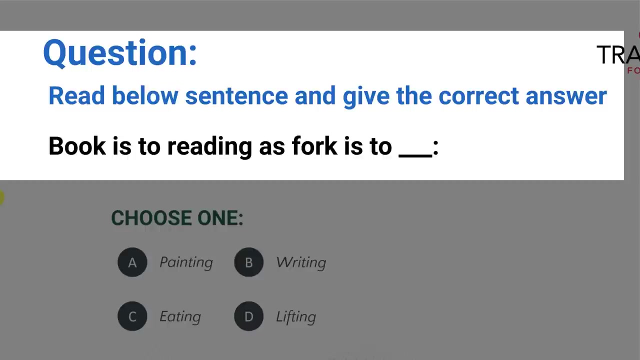 of previous two numbers. Hopefully you've got this one right. Now let's look at the reasoning question, where you need to complete the sentence Read below sentence and give the correct answer- Book is two reading as fork is two- And then you need to pick one of the four choices. 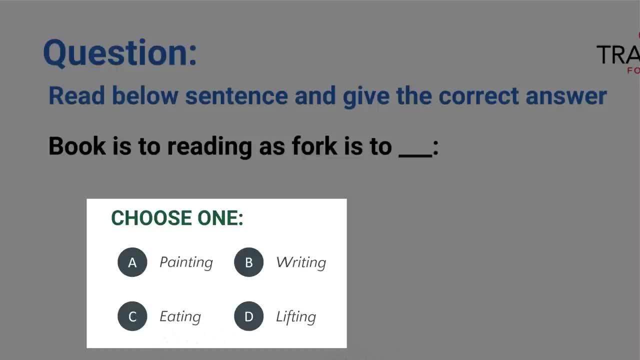 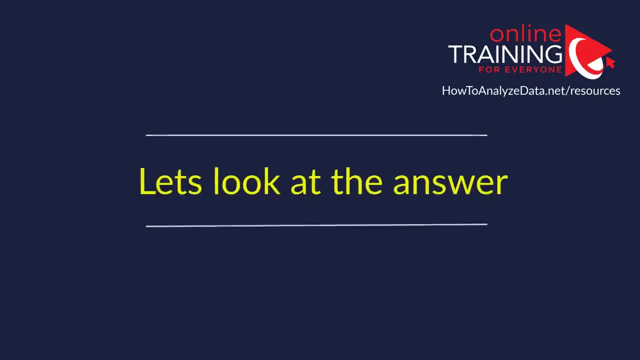 Painting, writing, eating and lifting. So what do you think is the right choice? I think it's pretty obvious here, So, but let's look at the right answer. So the correct answer is obviously eating right, Because book is two reading. 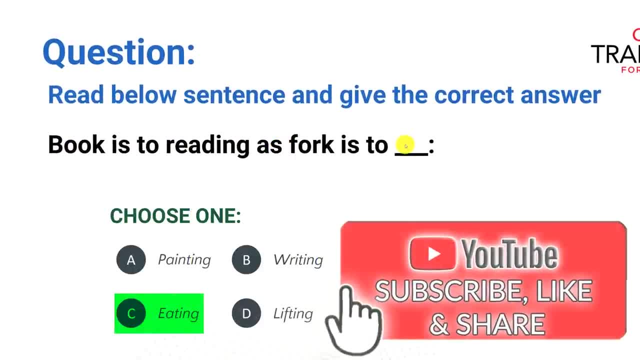 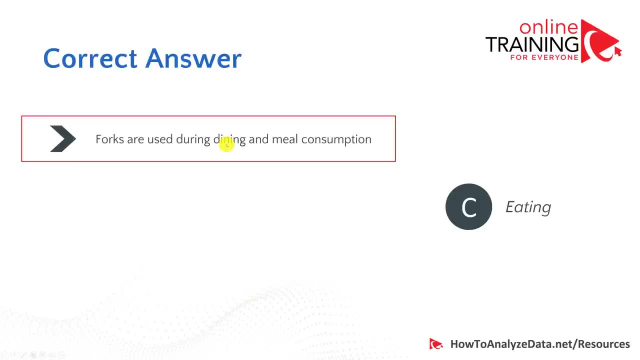 This is an activity associated with reading, As fork is two eating. You use fork during the meal consumption, So the correct choice is C, And that's because forks are used during dining and meal consumption. Hopefully you've got this one right Why you might consider subscribing to this channel. 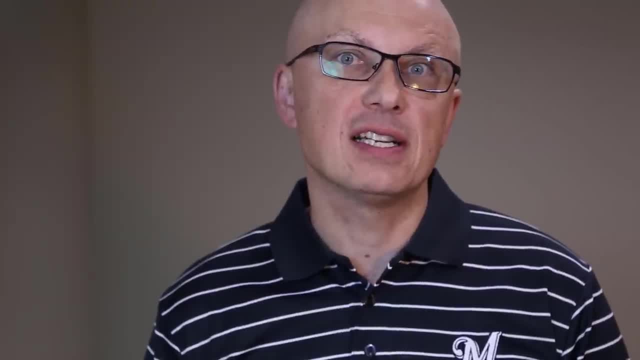 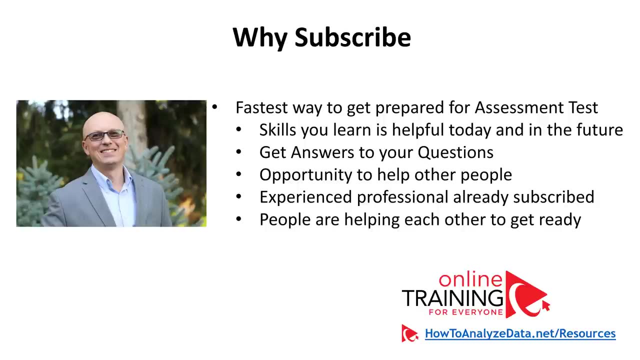 This is one of the fastest way to learn And get prepared for Excel assessment test. Skills you learn are helpful today and in the future. You get answers to your questions, You have opportunity to help other people And you have experienced professionals who already subscribed to this channel. 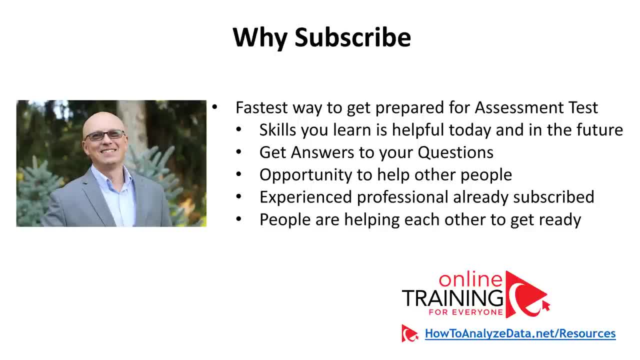 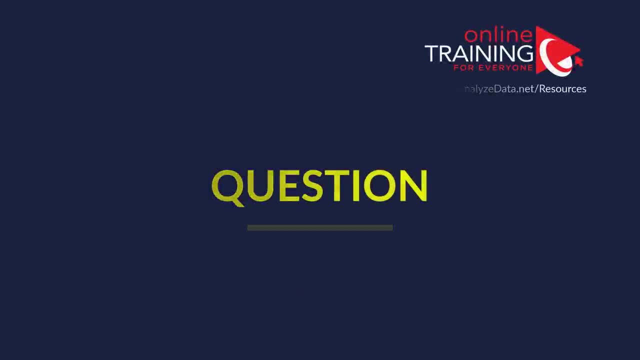 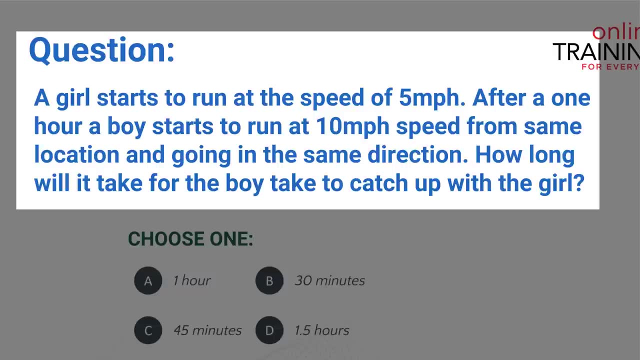 And ready to help you with any answers that you need. And now let's continue and get you ready for the test. Now let's look at the question which tests your knowledge of numerical reasoning. A good question. A girl starts to run at the speed of five miles per hour. 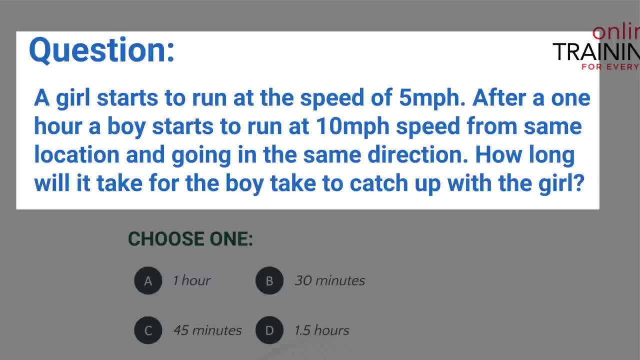 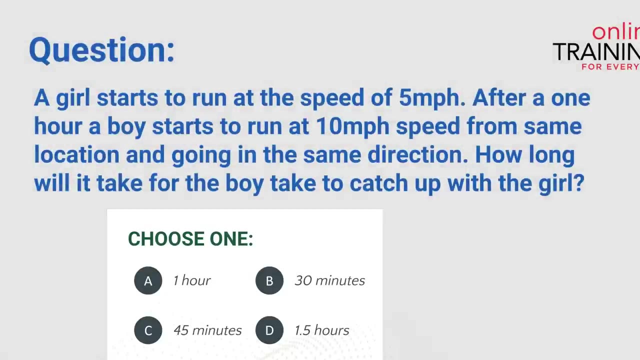 After one hour, a boy starts to run at 10 mile per hour speed from the same location and going in the same direction. How long will it take for the boy to catch up with the girl? And we have four choices here: One hour, 30 minutes, 45 minutes, 1.5 hours. 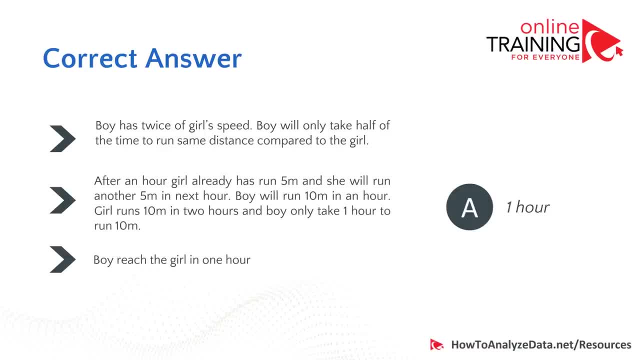 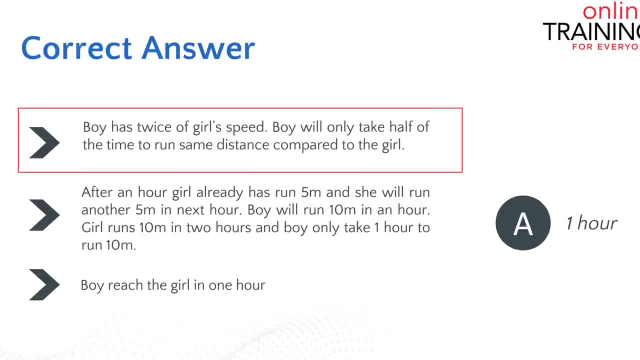 What do you think is the right choice? The correct answer here is A one hour, And here's the reasoning. Boy has twice of the girl's speed And for boy it will only take half the time to run the same distance compared to the girl. 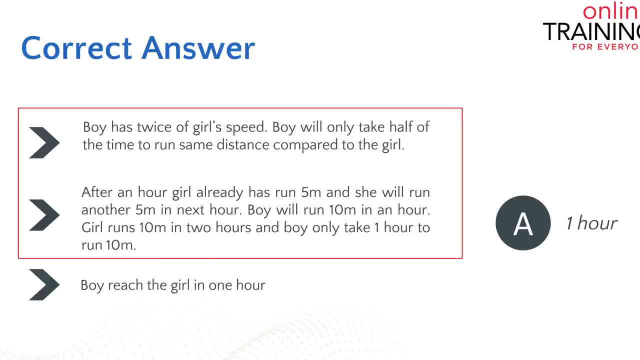 After an hour, girl already ran for five miles and she will run another five miles in the next hour. Boy, on the other hand, will run 10 miles an hour. Girl will run 10 miles in two hours, And for the boy it will take only one hour to run 10 miles. 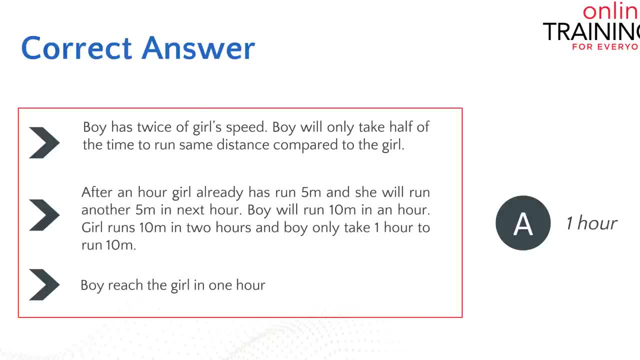 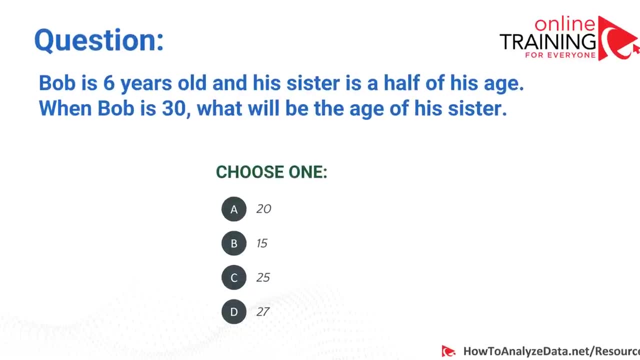 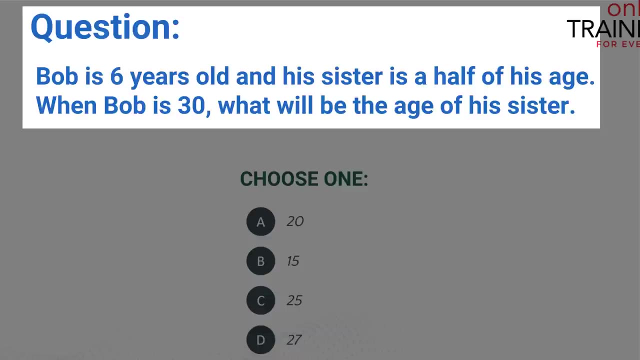 So boy will reach the girl in one hour. Hopefully you've got this one right. Here's another tricky question which can confuse you easily during the test. Bob is six years old and his sister is a half of his age. When Bob is 30, what would be the age of his sister? 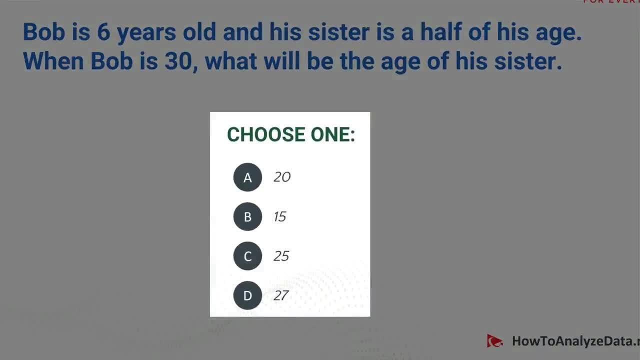 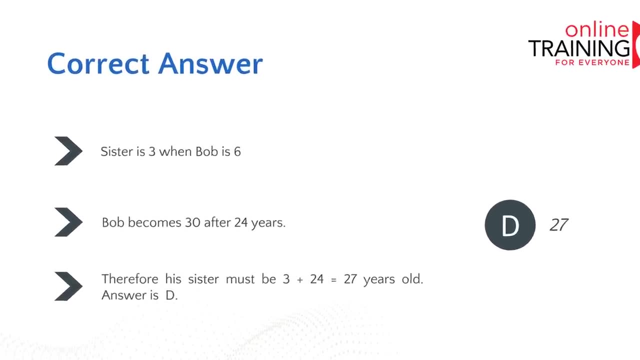 And there are four choices: 20,, 15,, 25, and 27.. Which one do you think is right? And obviously, as you might have figured out, the correct answer is D 27.. Bob's sister is three when Bob is six. 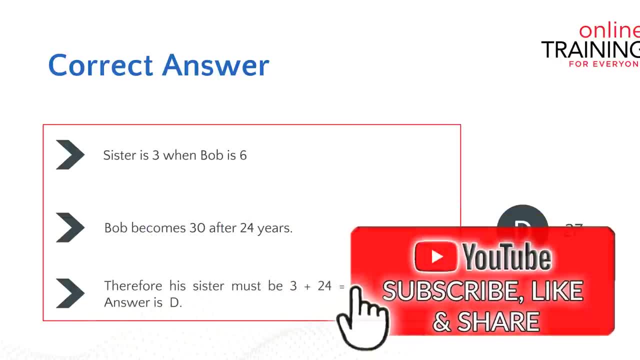 and Bob becomes 30 after 24 years, And Bob's sister is three when Bob is six and Bob becomes 30 after 24 years, And that's why his sister must be 27 years old And that's why his sister must be 27 years old. 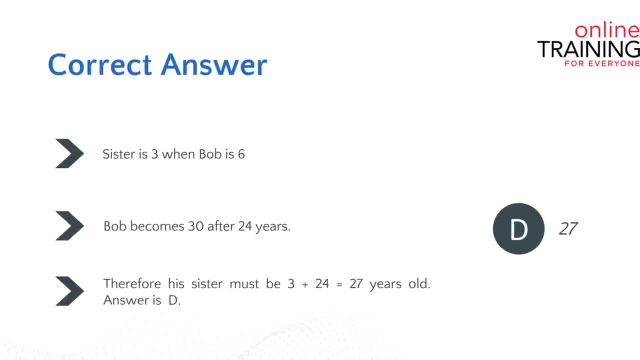 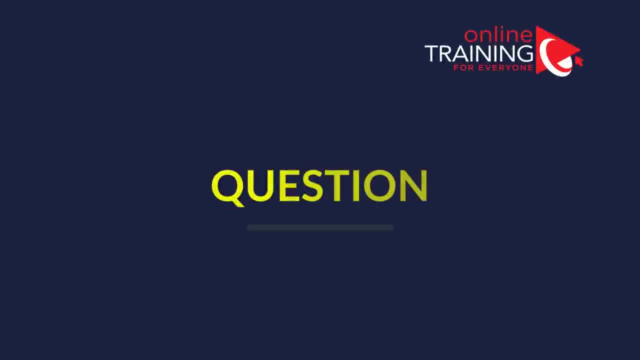 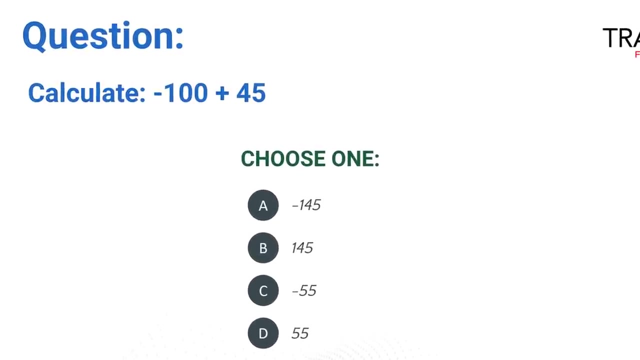 Another way to look at it. there is a three year difference. When Bob is 30, his sister would be 30 minus three, which would be 27.. Hopefully you've got this one right. Here's the question which tests your knowledge of working with negative numbers. 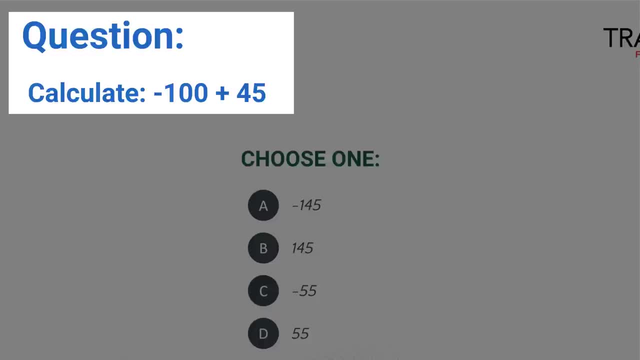 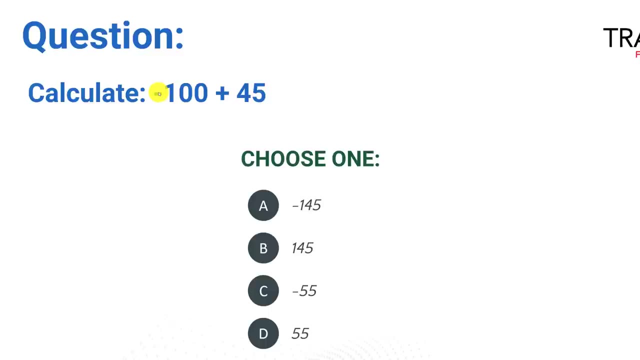 Calculate minus 100 plus 45. Here keep in mind that minus 100 is very tricky. Here keep in mind that minus 100 is very tricky. people just don't see this minus sign right before the 100. and there are four choices: minus 145, 145. 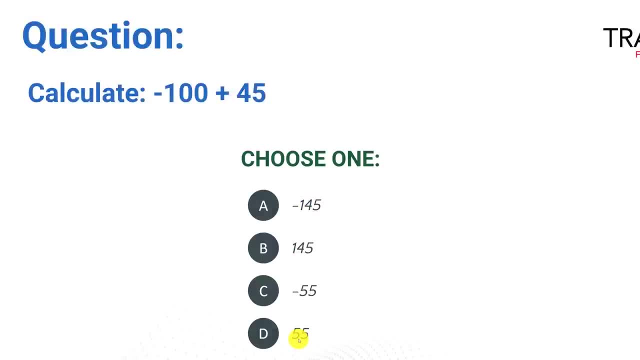 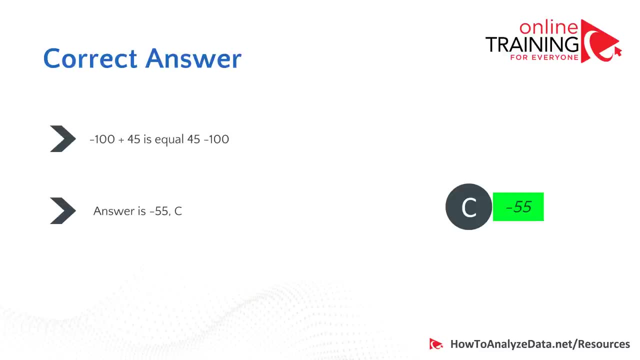 minus 55 and then 55. so what do you think is the right answer? and obviously the correct answer is c, which is minus 55, and the way we calculate this equation is we can move minus 100 after 45. so the new equation might look like this: 45 minus 100, which would be exactly minus 55, hopefully. 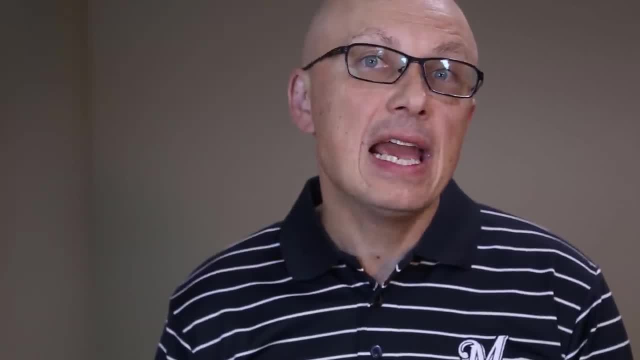 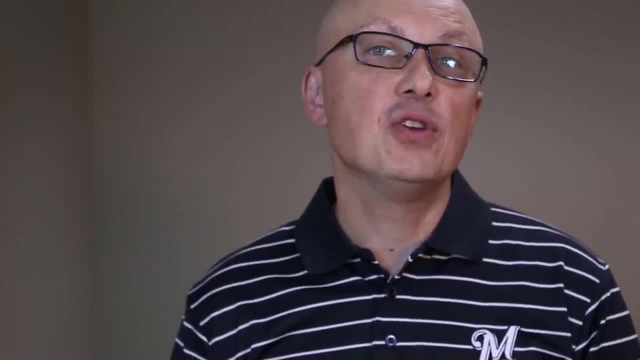 you've got this one correctly as well. a lot of people ask: how can I help on this channel? one of the best ways to help is to help other people answer the questions that they're getting. if you know the answer to the question that you see in comments, please post the answer in the comments. 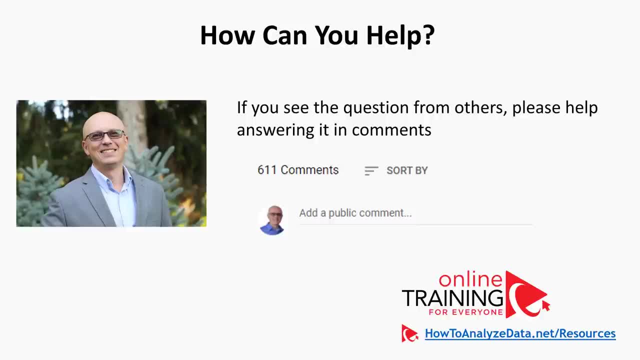 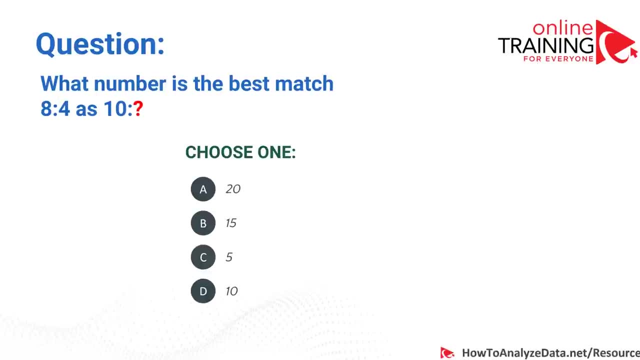 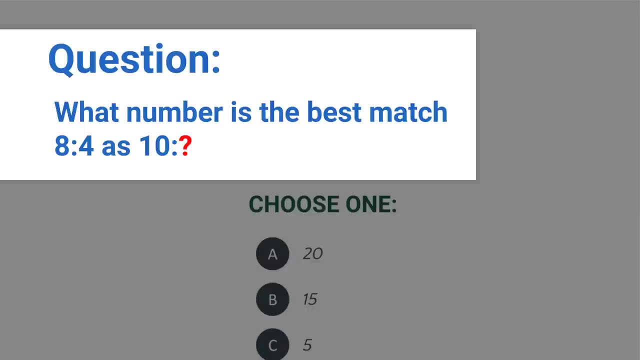 section of this video. and now let's continue and get you ready for the test. so let's look at another tricky question: what number is the best match? and we have eight to four would be 10 to question mark. so what do you think is the right one here? 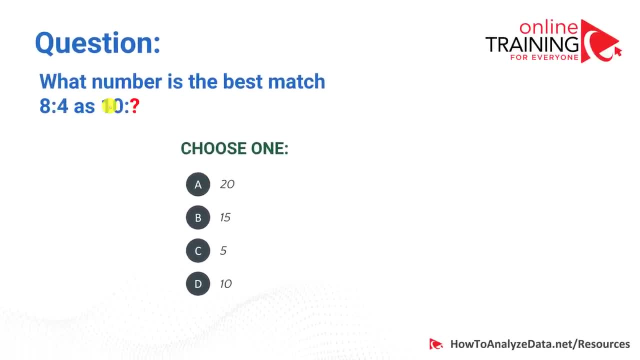 let's look at the answer. the best answer here is four is the half of eight, so the question mark would be half of 10, and in that case half of 10 is five, so that's the number you should choose. now the tricky part of this question: some people may mistakenly select 20, which would be double of 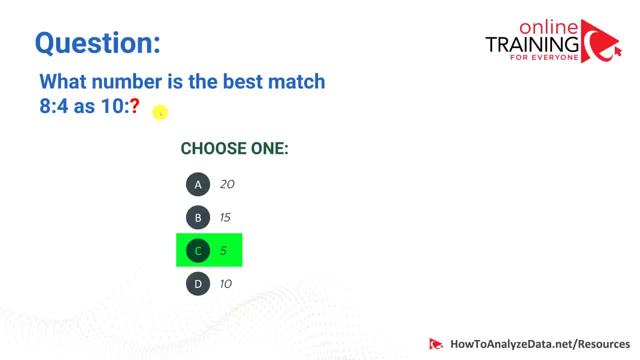 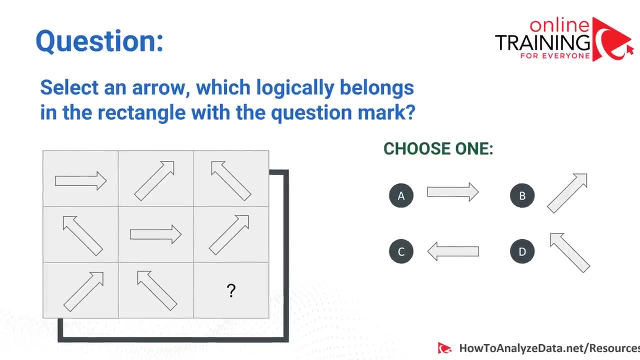 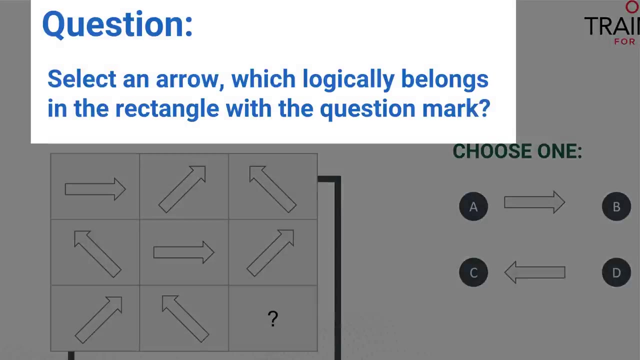 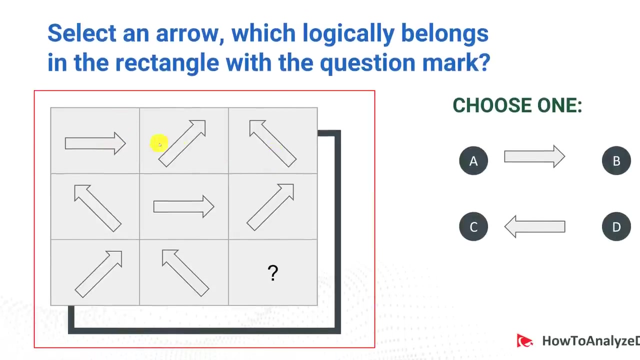 10. um, now let's look at the question which tests your knowledge of working with shapes, patterns and numbers. select an arrow which logically belongs in the rectangle with the question mark. here on the screen you see 3x3 box. each row of the box, in each column of the box, has arrows, one arrow. 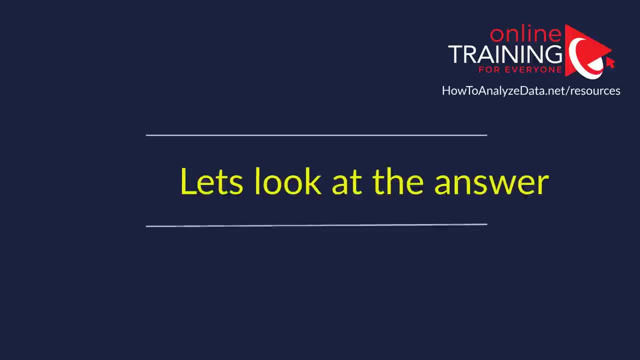 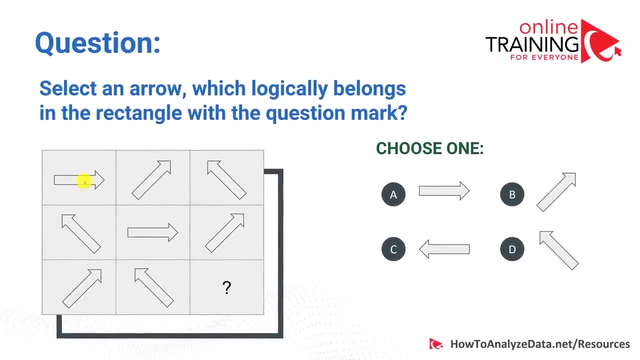 is missing. Which arrow do you think is missing? The key here is to identify the pattern. Each row and each column contains unique arrows. In the first row, we have arrow pointing to the right, upper right and then to the upper left, Then upper left, right and upper right. So here. 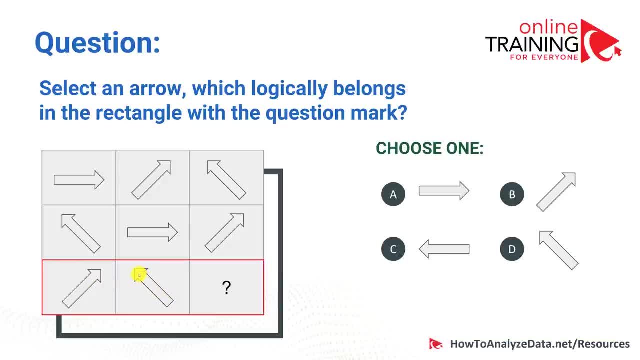 we have upper right and then we have arrow pointing to the upper left, And what's missing is the arrow pointing to the right, And that would be the right answer. And the arrow pointing to the right would be choice A, And this is the explanation. So each row has three arrows. 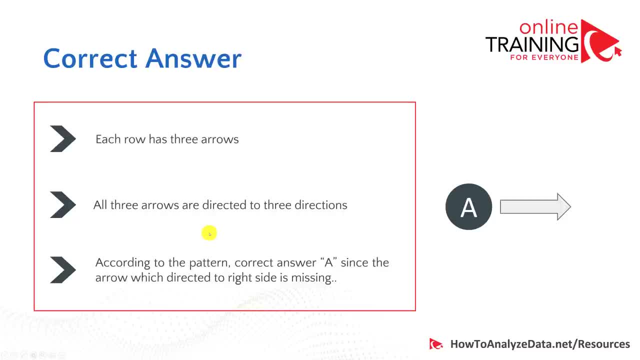 All three arrows are directed to three directions And they are unique. According to the pattern, correct answer is A, because arrow which is directed to the right is missing in the third row. Hopefully you've got this one right. So can you tell us? how many questions did you? 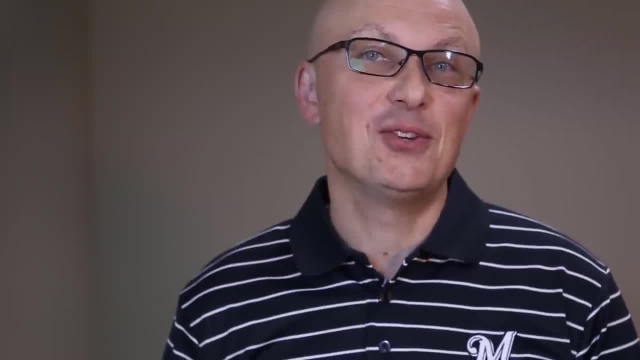 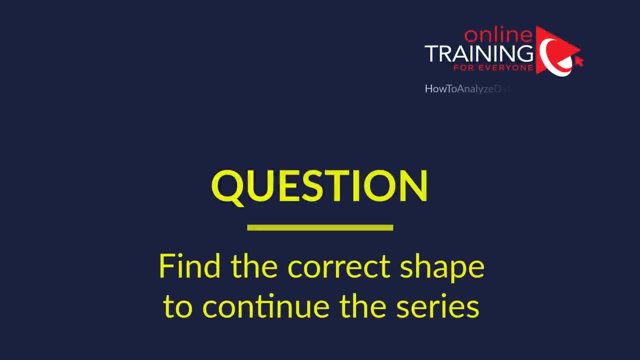 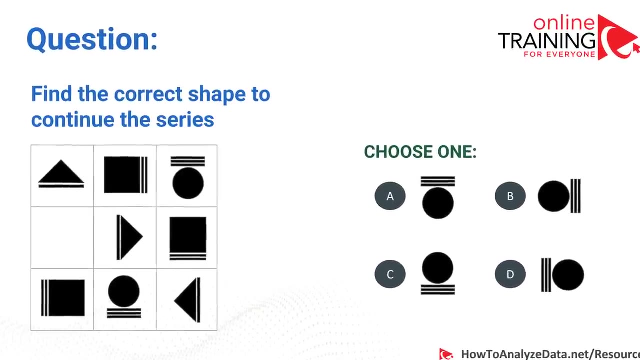 answer correctly. Please post in the comments of this video to share with others. And now let's continue and get you ready for the test. Now let's look at the very complex question which you see a lot during logical reasoning tests, psychometric tests and the numerical reasoning tests. Find the correct shape to 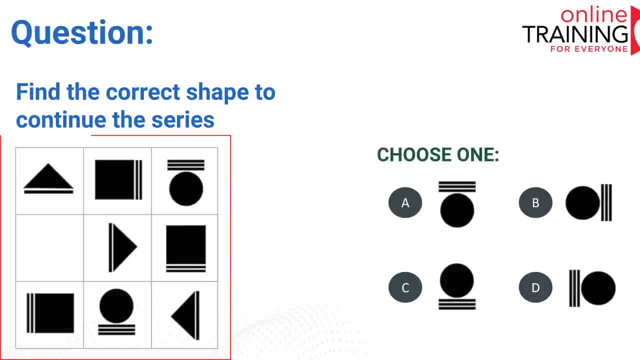 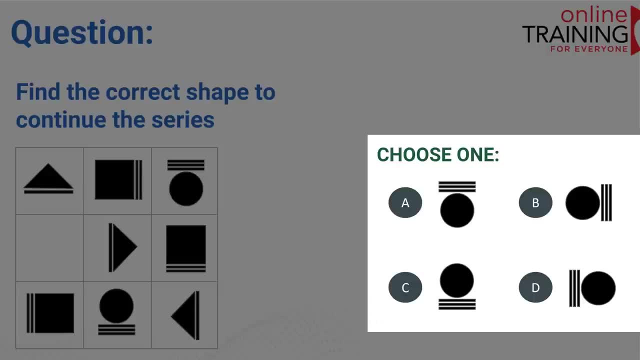 continue the series And what we have here? we have three by three matrix with eight shapes populated and one shape is missing. There are four choices, as usual, but in order for you to choose the right one, you have to choose the right one. So let's start with the right one. 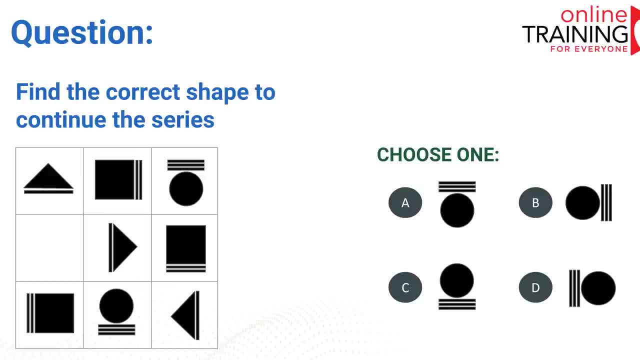 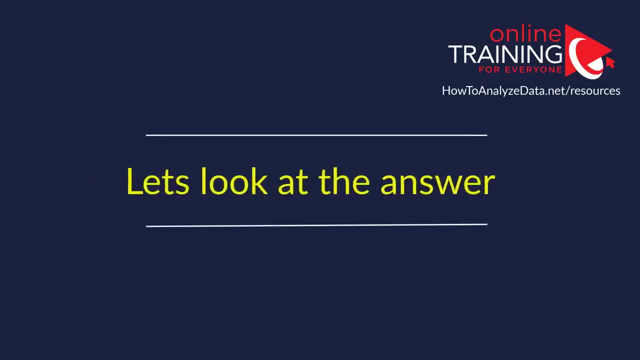 If you want to calculate the right shape, you need to determine the pattern, And in fact there are two patterns here on the screen. Can you figure it out? Do you know what the right answer is? As I mentioned, there are two patterns here. One is: there is a pattern for the shape Which? 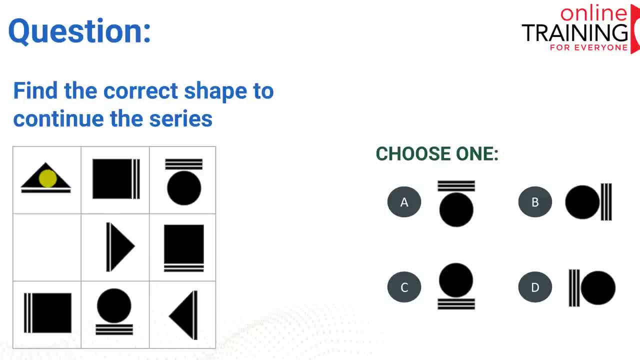 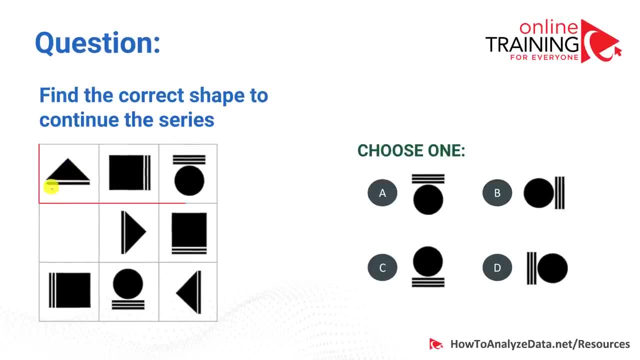 shape would you choose? And second, pattern is the pattern for the lines, And where is the right location for the line itself? Now let's go through the detection of the shape pattern first. So the shape pattern is triangle, square, and then the circle right. So triangle, square and then the 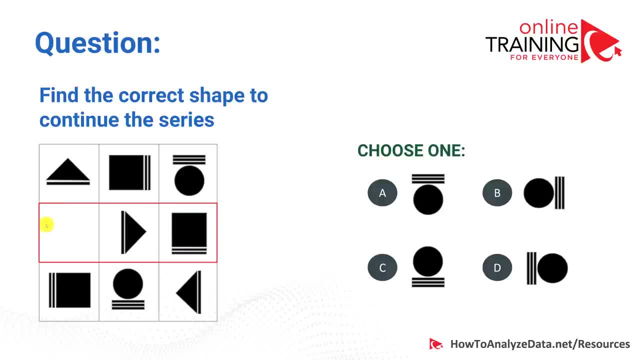 next one would be the circle. So we have a circle- that's the right value here- but all of this, other circles. So this was helpful, but not by much. But it just tells us that we are detecting the first pattern And here, if you want to confirm, we have square circle and then triangle. Now 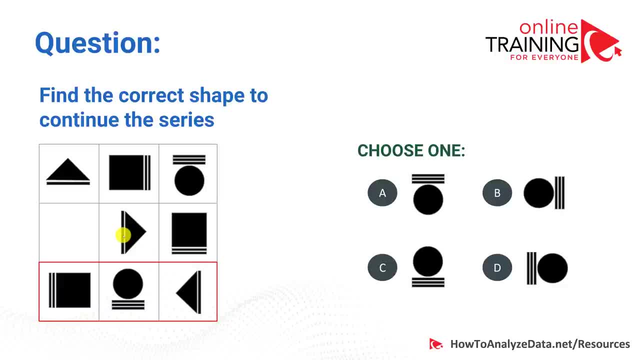 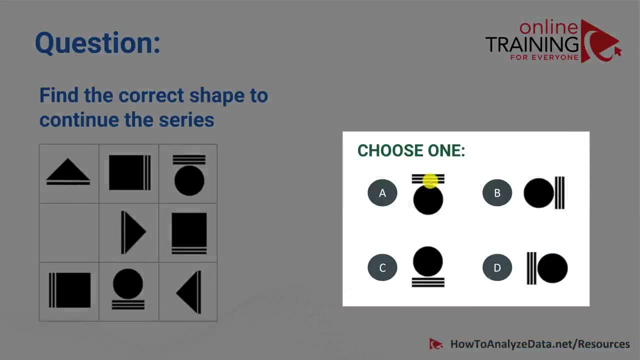 the most important part here is to determine on which side of the shape the lines should be located, And what we have here. we have four locations, as you can see in the answer: One location on the top and then the other location on the left. So we have four locations and then 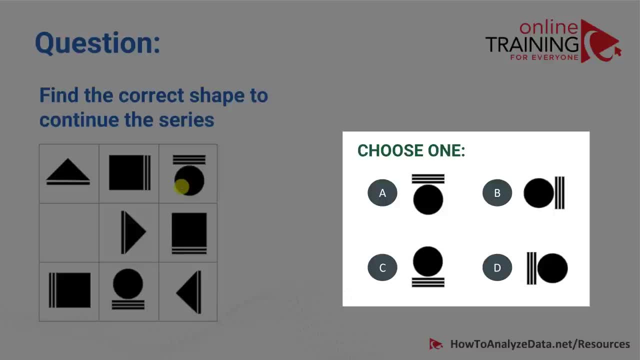 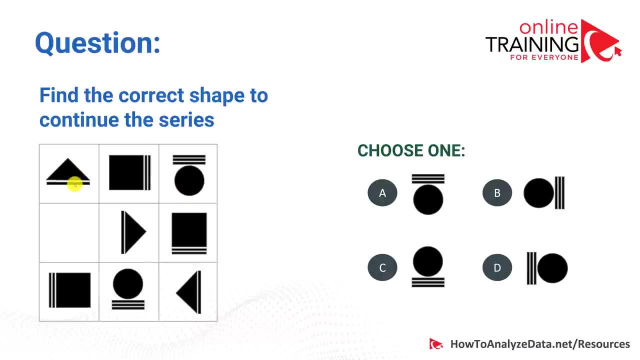 the other location on the right, left and bottom. So how would you know where is the right location for the circle shape? So let's look closely here and let's detect the pattern here for the line location. The line location starts with the bottom, right and then top. So you see. 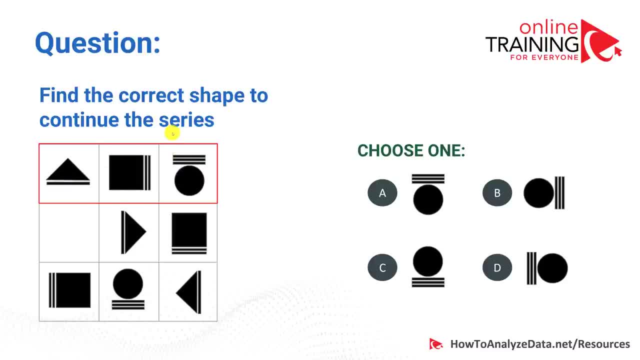 it's going counterclockwise. So if you imagine the clock with the clockwise rotation, then this would be counterclockwise. And let's see if we are correct and we have a pattern here. So we have bottom right, top, Then we have left bottom, So that still matches the counterclockwise pattern. 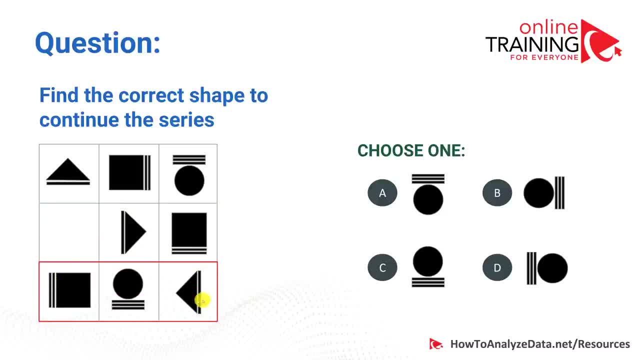 And then we have left, bottom right. So I think the missing shape here would be the one before the left, which would be on the top. So the right answer in this case would be A, because here we have a circle which matches the circle's pattern, And then we have lines located at the top. Let's 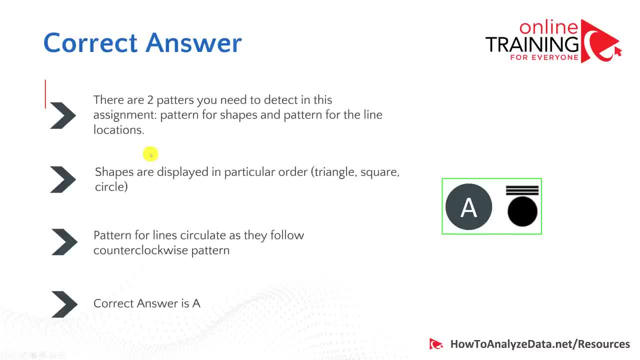 verify, to confirm that And, as you can see, the correct answer is A. So let's recap. There are two patterns you need to detect in this assignment: Patterns for the shapes and pattern for the line location. Shapes are displayed in a particular order Triangle. 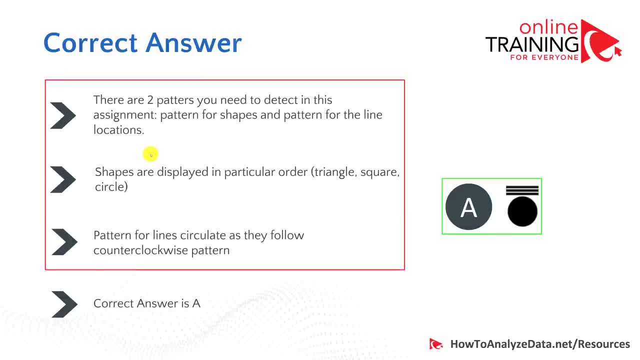 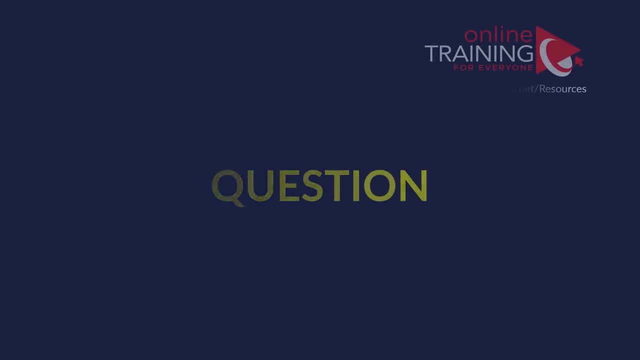 square circle. That's really the pattern for the shapes And pattern for lines are in a counterclockwise order, So correct answer is A. Hopefully you've got this one right. You will see a lot of these types of questions in the assessment test. Let's look at the question. 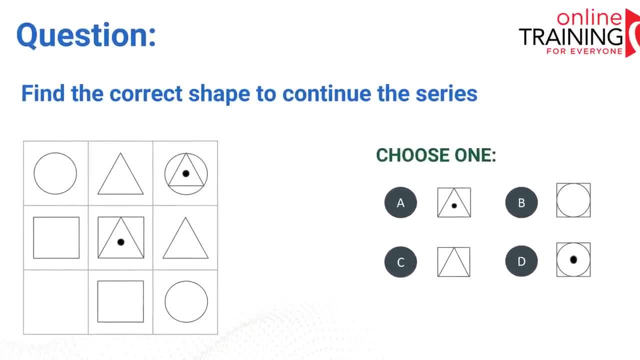 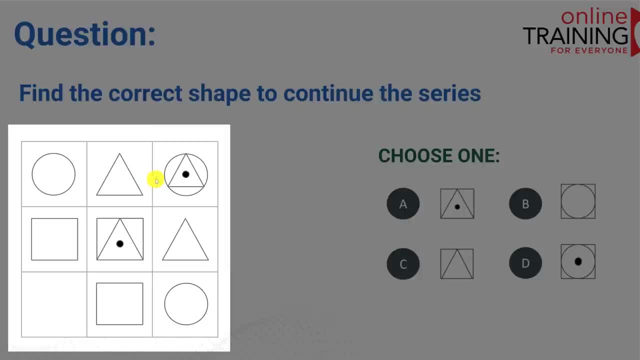 which is frequently used in the assessment test. Let's use this part of numeric reasoning test, an aptitude test. Find the correct shape to continue the series And you're presented with the 3x3 box, which contains multiple shapes, and one shape is. 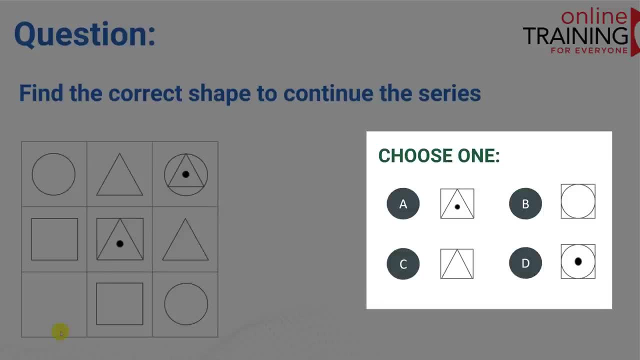 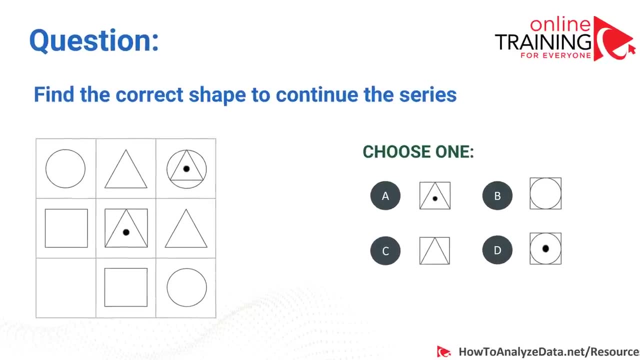 missing in one of the boxes. There are four choices. Can you detect which one is the correct one? Before I jump to the final answer, let me teach you how to detect patterns in these types of questions. There are three different patterns that we can see here. First pattern is pattern in. 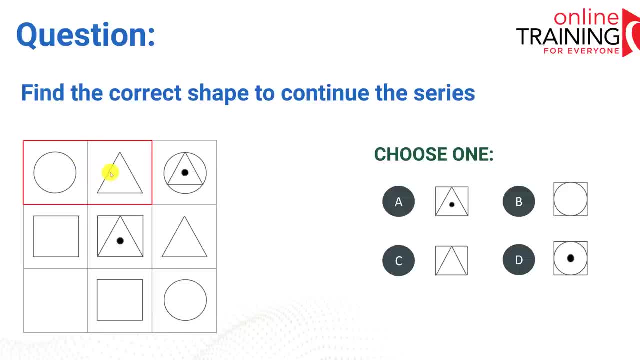 the shapes. We have circle, which is the shape of the line, and circle, which is the shape of the line. We have triangle and triangle in the first row, We have square and triangle in the second row, And then we have square and circle in the third row. The second pattern here is the pattern. 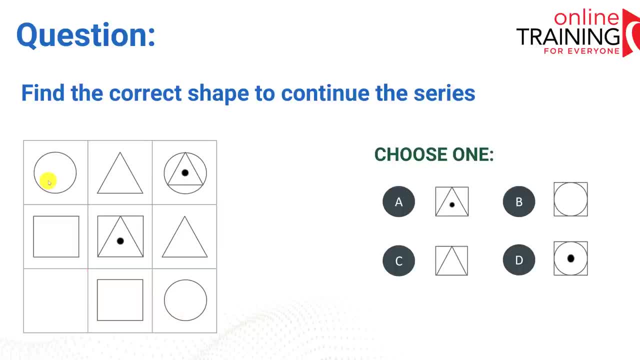 of one shape inside of the other. So what you see here is that every row contains one shape inside of the other. In the first row, it's a triangle inside of the circle, In the second row, it's the triangle inside of the square, And the third one is missing. this pattern which tells us that it. 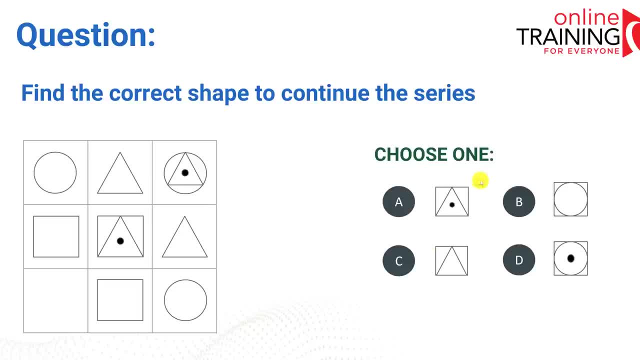 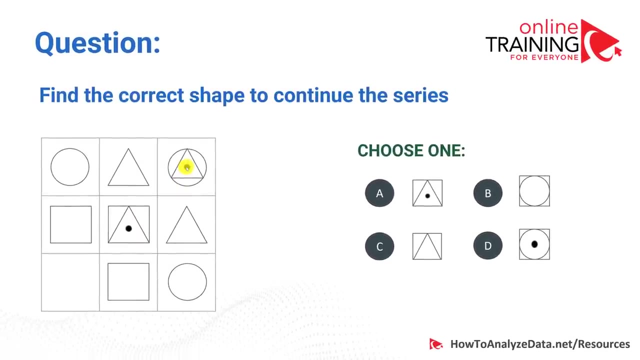 should be the pattern of one shape inside of the other, Which is not true. So let's look at the third pattern. And the third pattern is the dot in the middle of the shape. So you see that every row contains at least one shape, where dot is inside of the shapes that are one inside of the 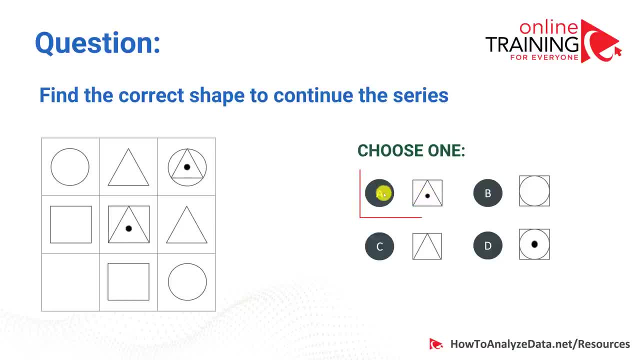 other. So, knowing this information, we have our choices A and D, because we narrowed it down and recognize that we have one shape inside of the other. So let's look at the third pattern, And the third pattern is that we have to have a dot inside of the shape. Now, which one do you think? 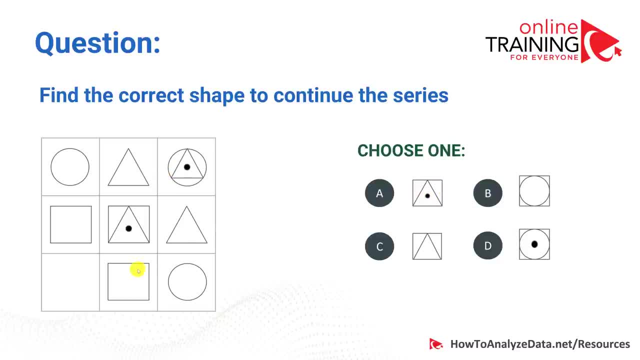 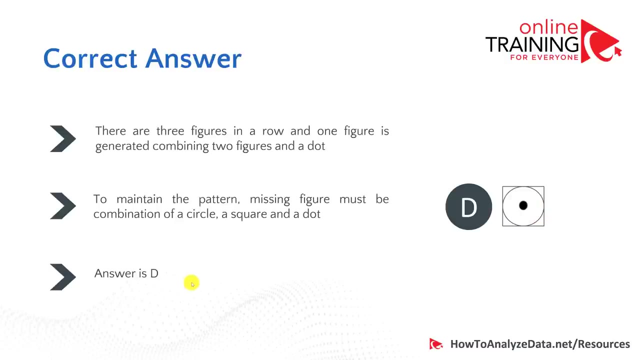 is right. Knowing the first pattern, we can exclude choice A because in the third row we have combination of squares and circles. So the correct choice is D because it matches all three patterns. We have circle inside of the square and then we have dot in the middle, So the correct answer is: 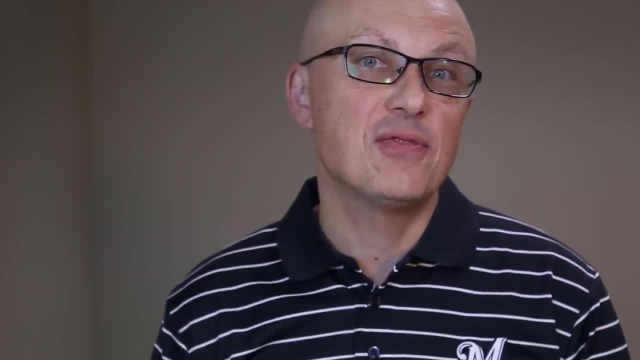 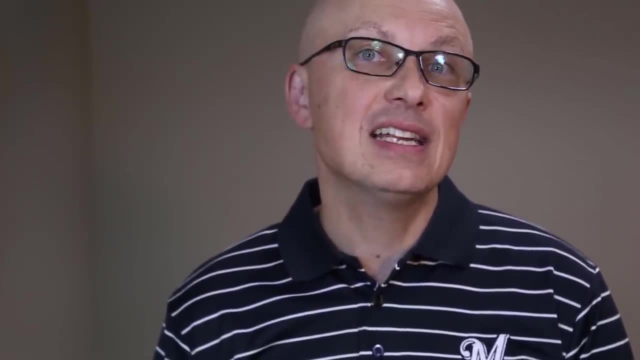 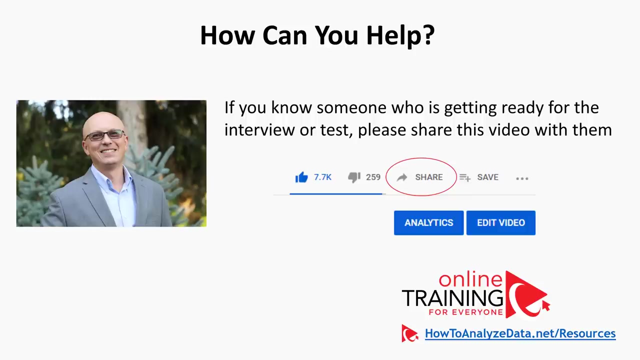 D. Hopefully you've got this one right. Can I ask you to do me a favor: If you know someone who is getting ready for interview or Excel assessment, please let me know in the comments below. And now let's continue and get you ready for the test.